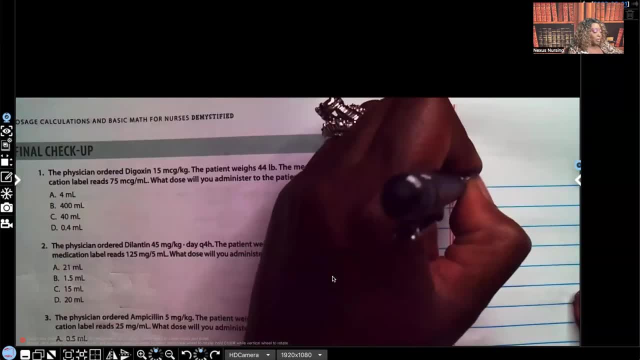 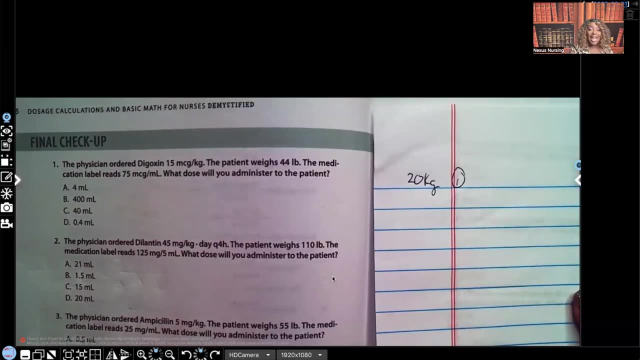 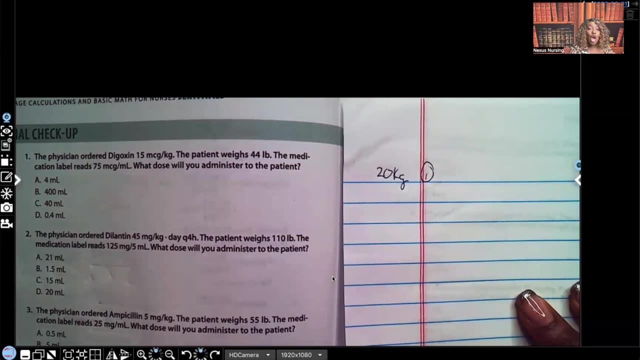 kilograms. So I'm going to write my 20 kilograms right here: 20 kilograms, So I don't forget, My patient weighs 20 kilograms. Now that I have my patient's kilograms, I can get started on this problem. How am I going to set it up? Always start with what you have. What you have is what you have. 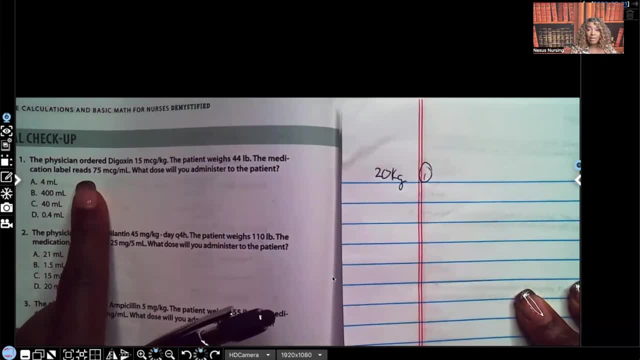 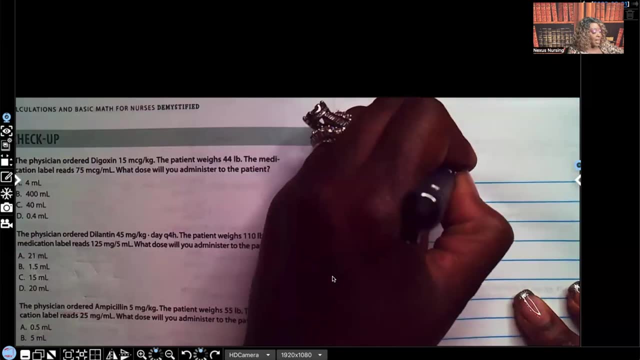 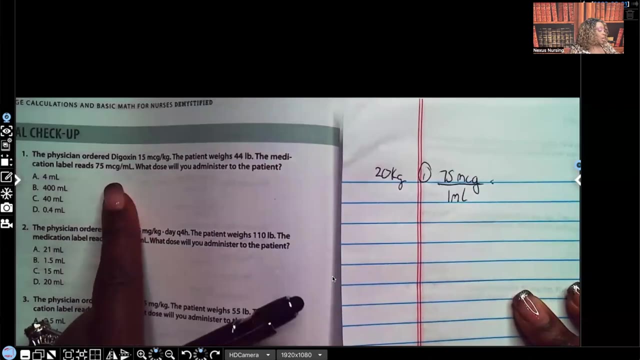 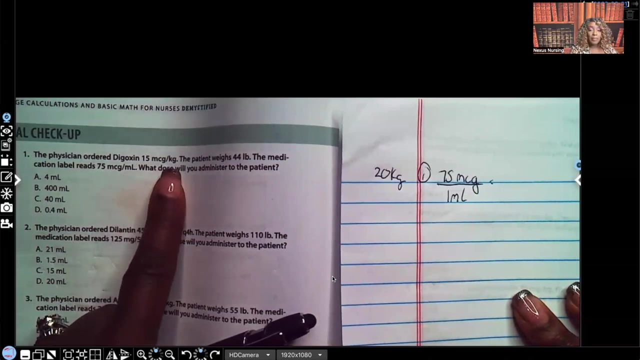 So always start with that, And what we have is what the label reads. The label is what you have on hand. It's 75 micrograms per ml, So write that down: 75 micrograms per 1 ml. Okay, What is the order? The order is: digoxin: 15 micrograms per kilogram. All I have to do is 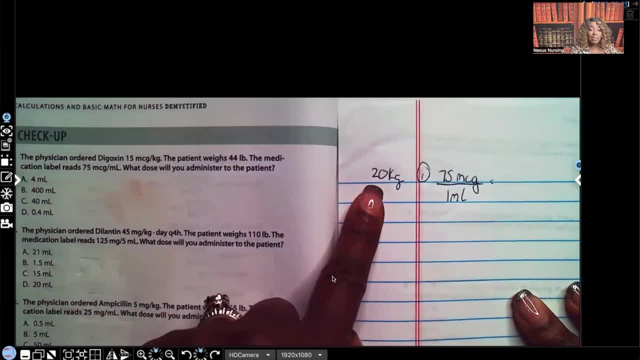 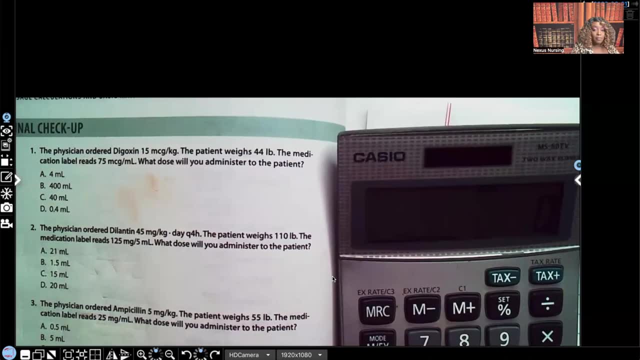 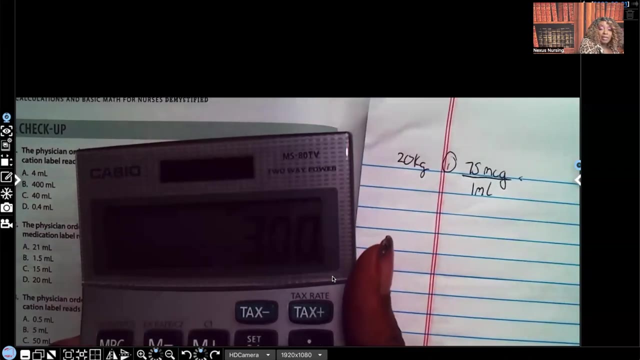 multiply that micrograms times my kilograms. I have already. So I do 15 times 20.. Pull out my calculator, Let me try. I'll do it under the light for you: 15 times 20. And that gives me 300.. See that 300.. So that means I'm going to be giving 300. 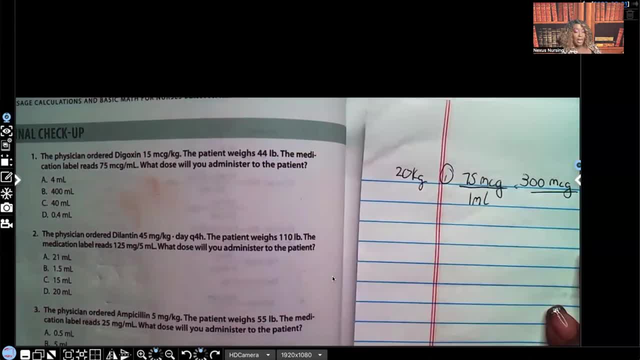 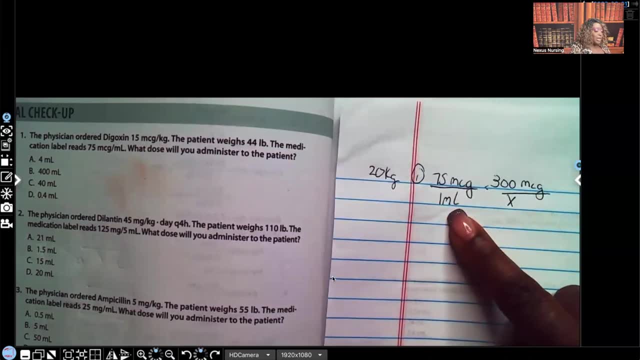 micrograms. And what do I have down here? X, X is what we're solving for Microgram, microgram, milliliter. So my X is going to be milliliters, because my units always have to match. What's the next step? 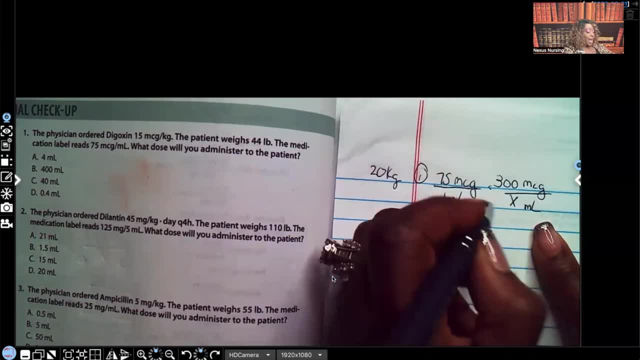 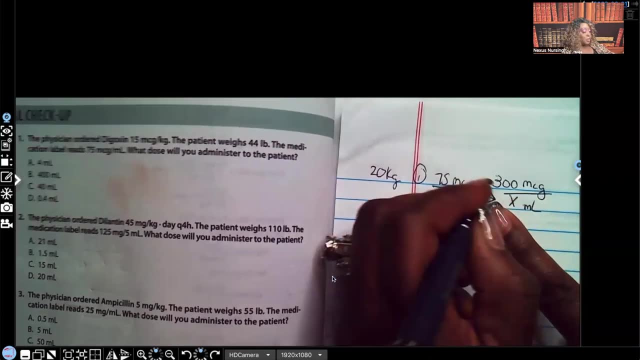 After I've set up my equation, I'm going to cross, multiply, I'm going to do 75 times X, which gives me 75 X, And then I do 300 times 1.. I have to cross, multiply 300 times 1,. 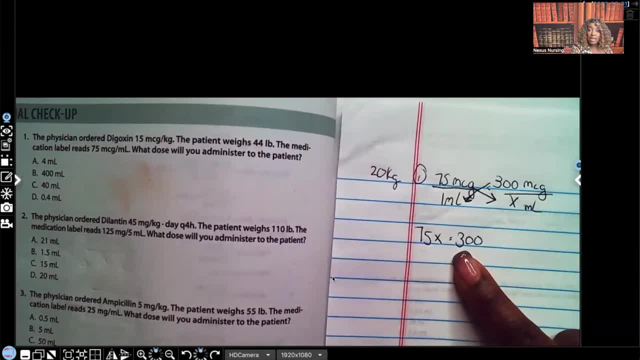 which gives me 300.. Now I have 75. X equals 300.. I have to get X by itself. Remember, that's what I'm solving for. So how am I going to get X by itself? Divide by both sides. Divide by. 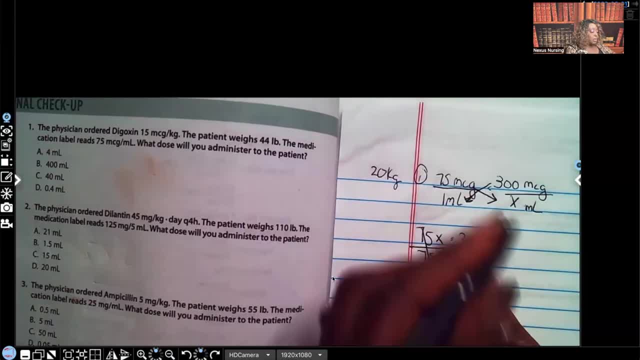 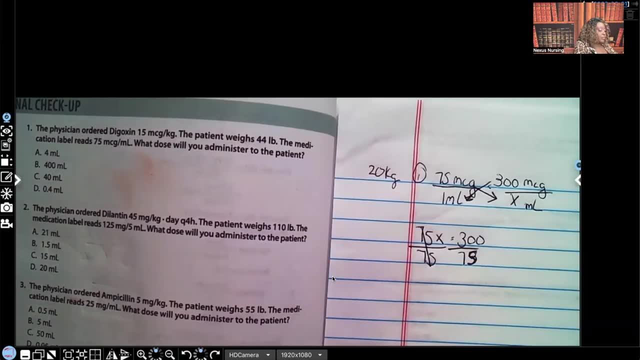 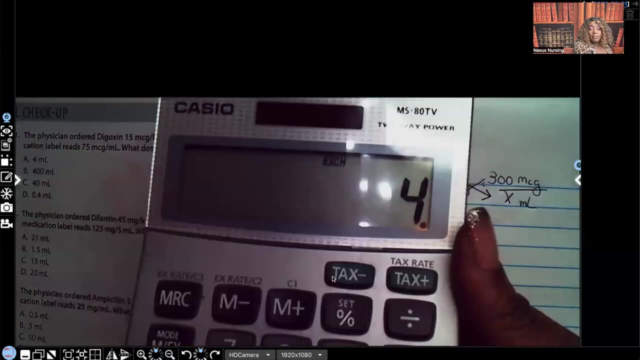 75.. Divide by 75.. Oop 75.. How many times does 75 go into 300?? I have no clue. Let me pull out my calculator Four. See that Four. So my answer is four. But am I done If I just leave it like this? 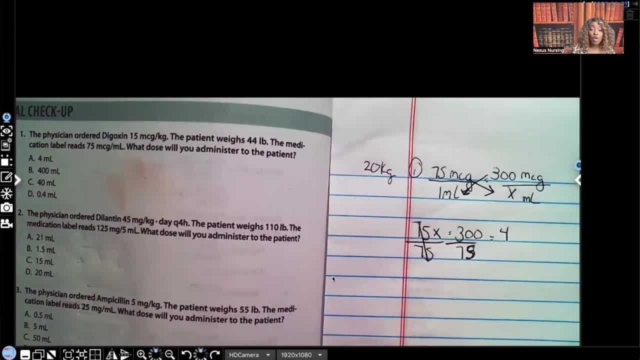 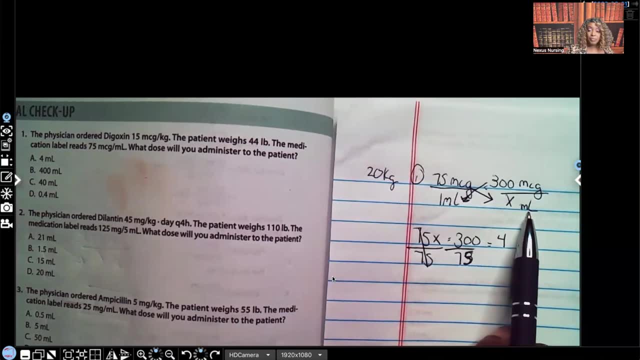 is it going to be correct? Absolutely not. You always have to have your unit of measurement. If you forget what your unit of measurement is, go back to X, because that's what we're solving for. And when you look, it's ML. So I'm giving four. 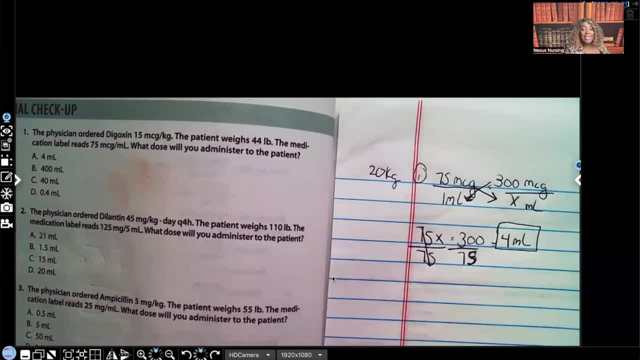 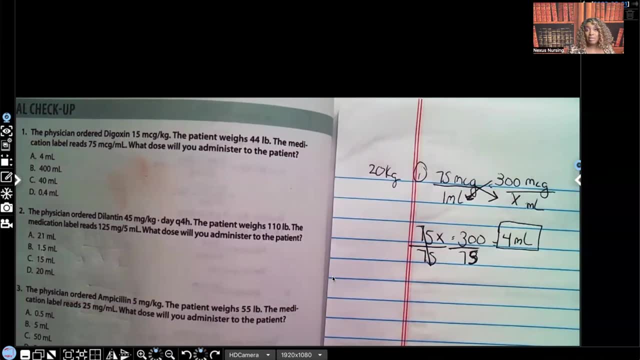 That is my answer: Four MLs. And that's why it's so important, when you're setting up your problem, always put your unit, Because if you don't, you might make a mistake and get confused. Okay, So let's do the second problem. 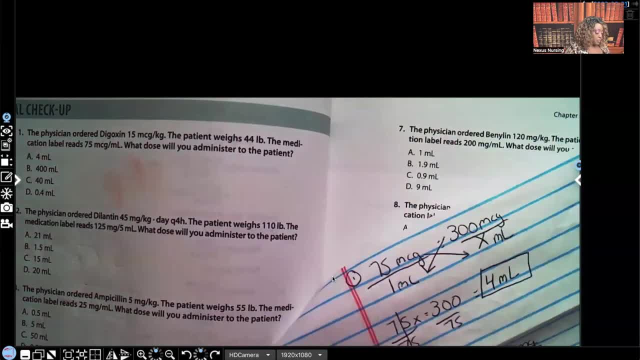 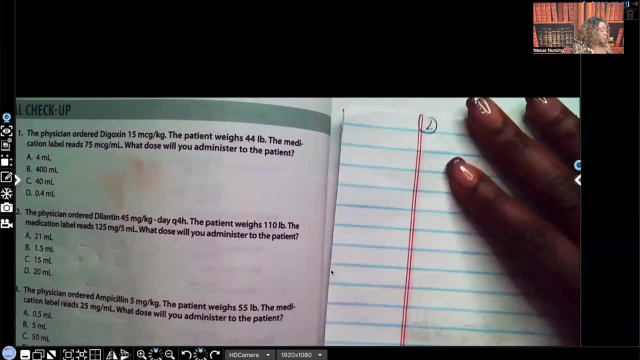 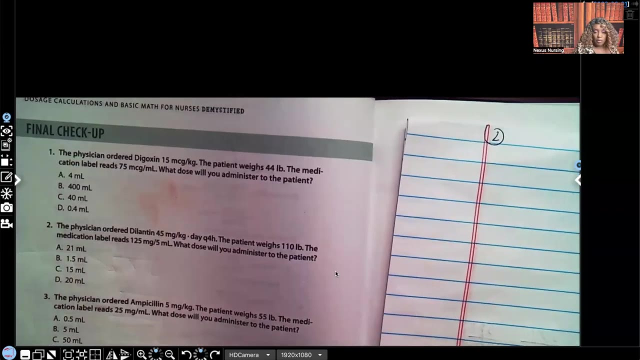 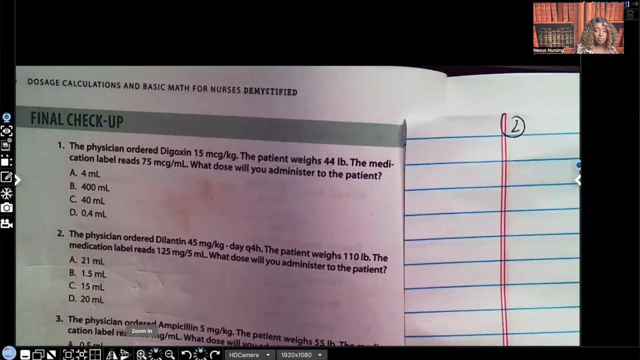 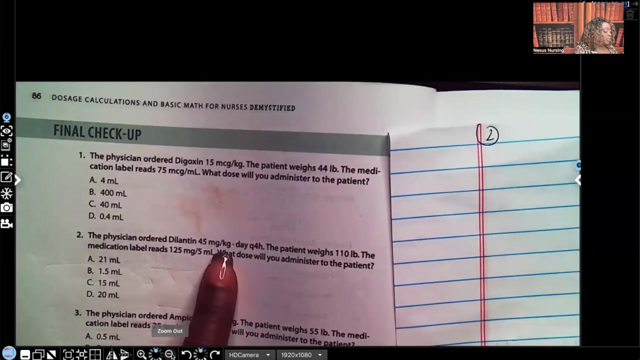 Let's do number two. Look at number two, My paper's dirty, but don't worry about that. It says: let me make this a little bit bigger for you. Okay. It says the physician orders Dilantin 45 milligrams per kilogram. per day, every four hours. the patient weighs 110 pounds. The medication label reads 125 milligrams per five MLs. What dose will you administer? Uh, to the patient. So, again, the first thing we want to do is turn our pounds into kilograms. 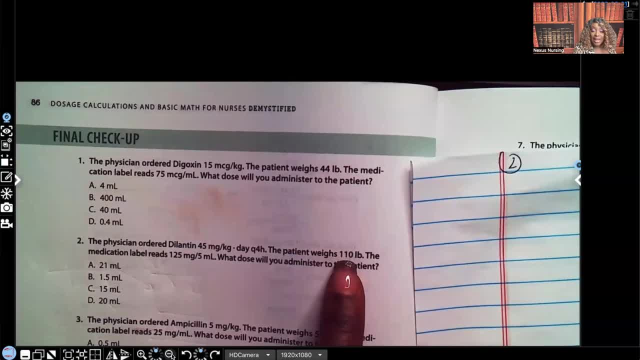 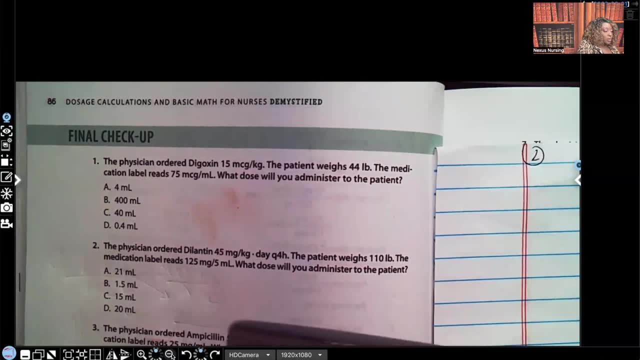 And you do that by dividing by 2.2, one 10 divided by 2.2. One 10 divided by 2.2. And that gives us 50. Okay, So let me write that on the side, So I. 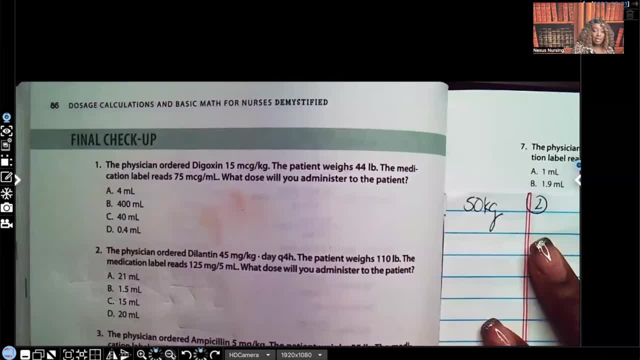 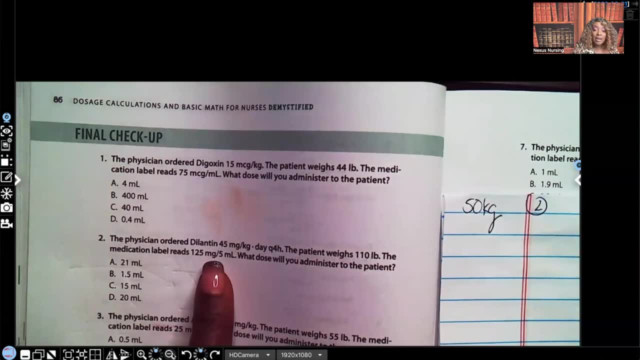 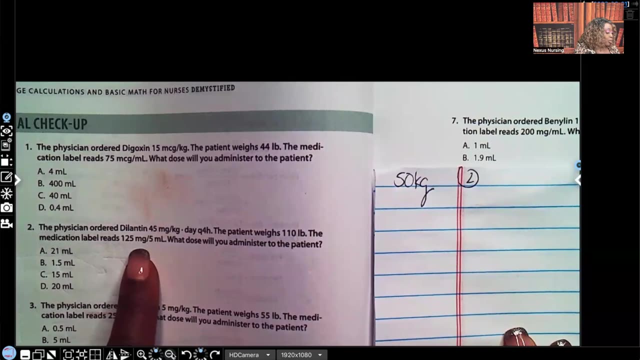 don't forget, my kid weighs 50 kilograms. This is how much my kid weighs. Next, we're going to set up our problem. Remember, we're always going to set up, starting with what we have. What we have is what is on the label. That's what we have, Okay, So the label reads: 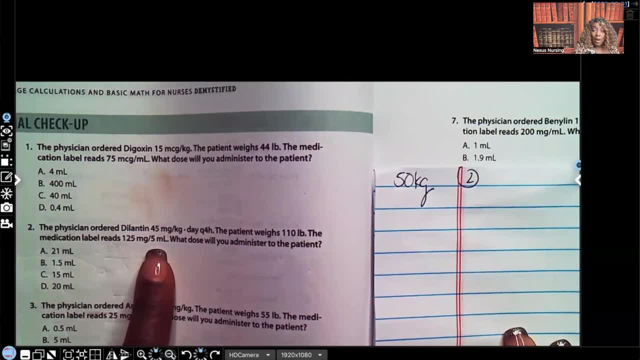 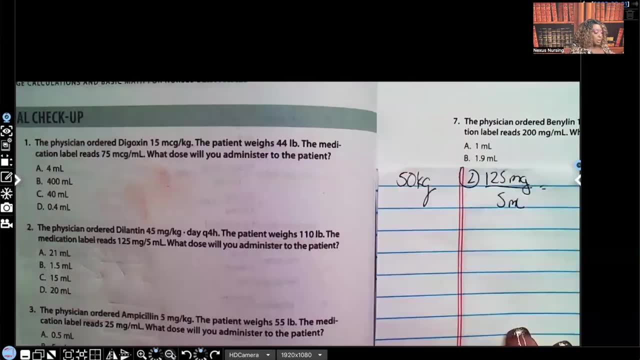 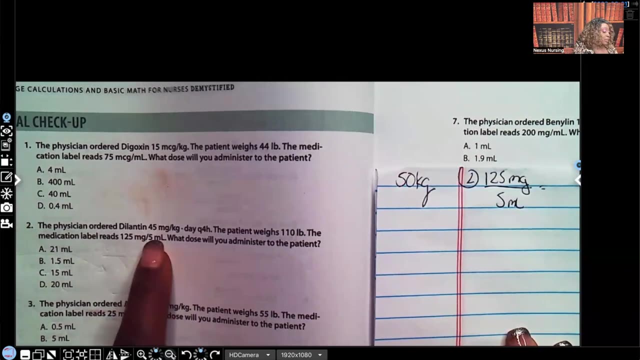 125 milligrams over five ML. write it down: 125 milligrams over five ML equals. Well, look at what's ordered: 45 milligrams per kilogram. So we have to do is multiply that milligram, which is 45 times our kilogram, which is 50, 45 times 50,. 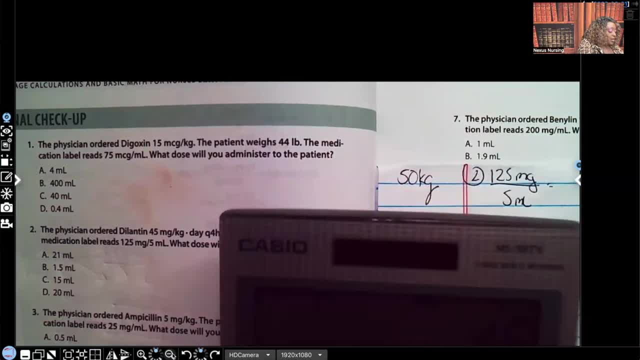 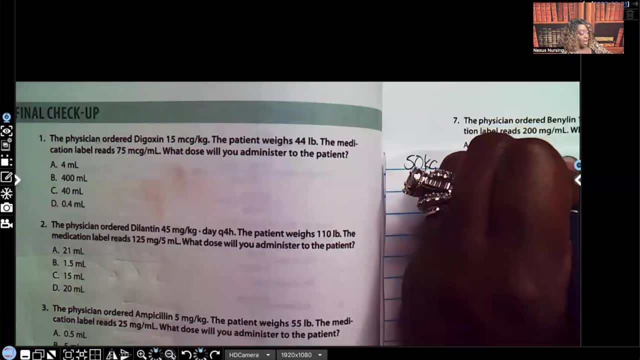 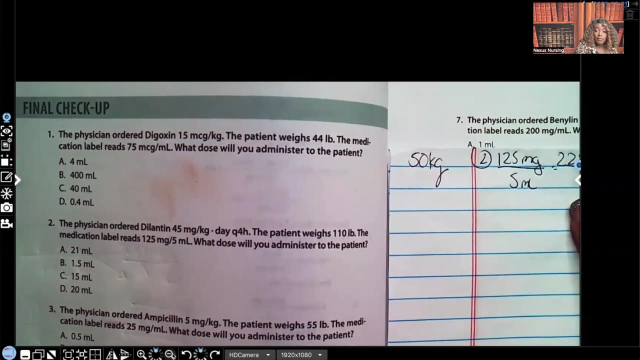 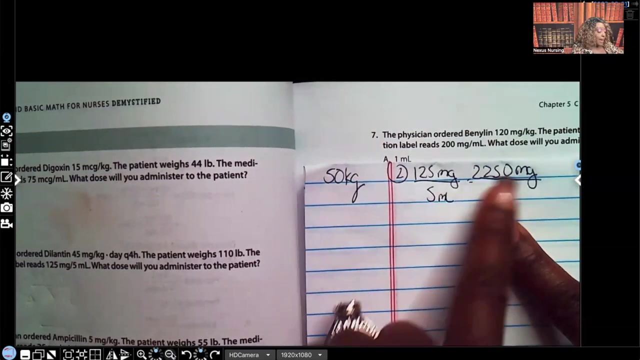 45 times 50. That gives us 2250.. So I'm going to give- write it down: 2250 milligrams right Over X. Remember, X is what we're solving for Your units have to always match Milligram, milligram, milliliters, X, what milliliters? write it down So you don't forget. 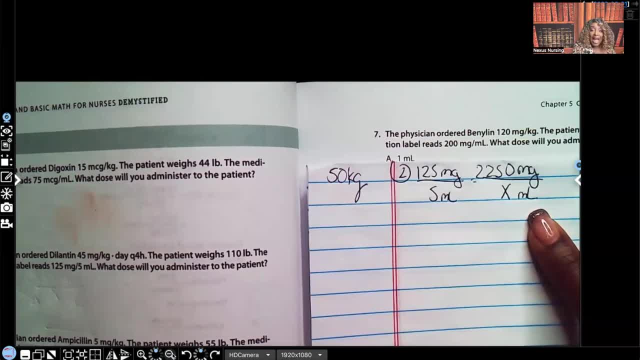 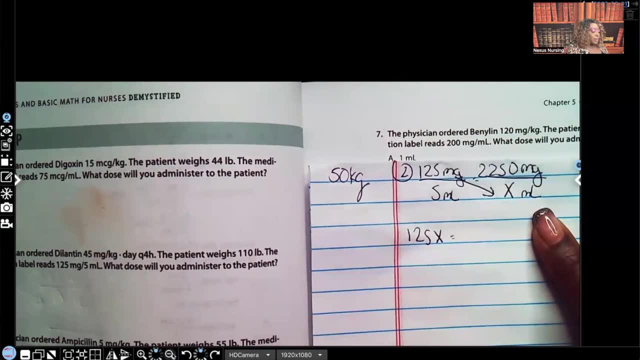 now that all of my units match, I can cross multiply. I'm going to multiply 125 times X, which gives me 125 X and 2250 times five. What is that? I have no idea. Let's plug it in the. 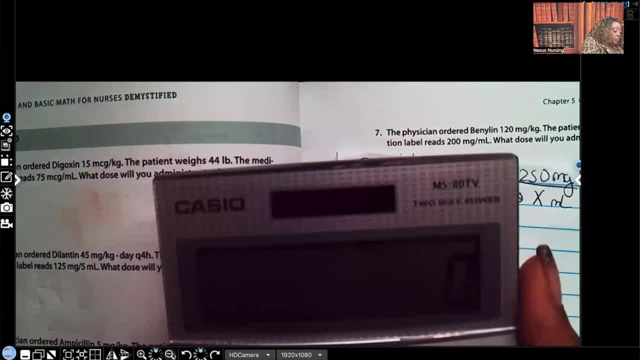 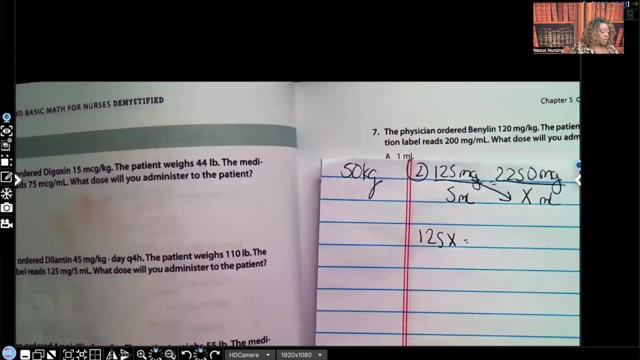 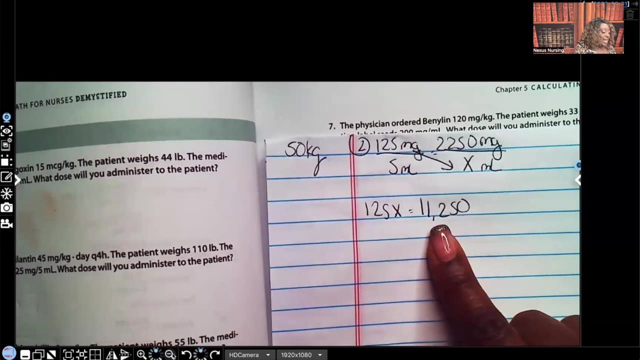 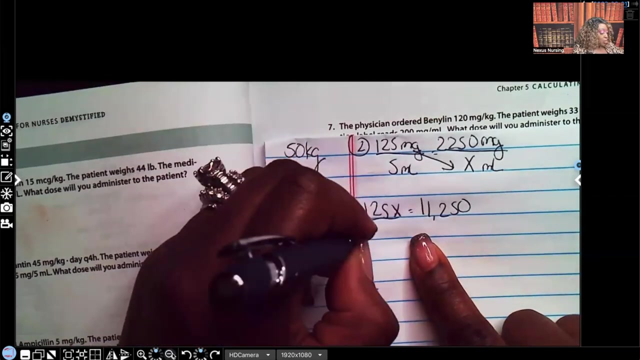 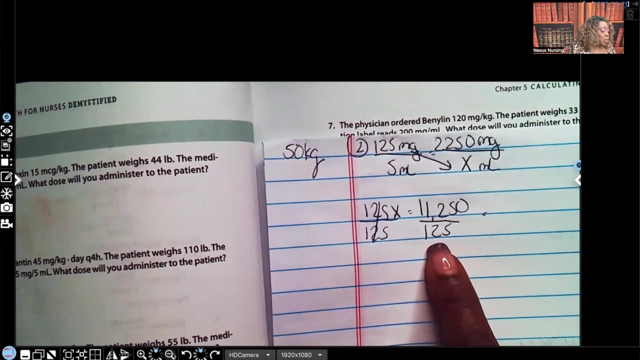 calculator: 2250 times five, That gives me 11.. 2250.. So write it down: 11,250.. So I have 125. X equals 11,250.. Again, I got to get X by itself. I'm going to divide by both sides, divide by 125, divide by 125. So um 125 goes into 11,. 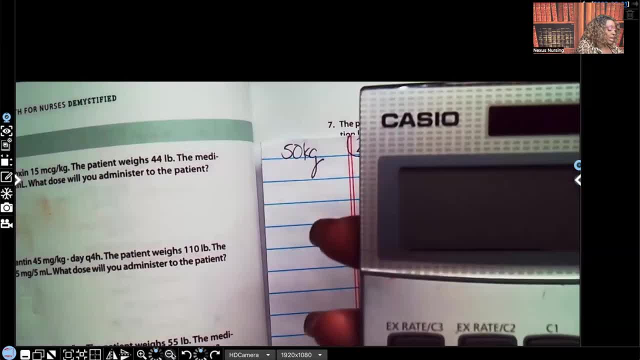 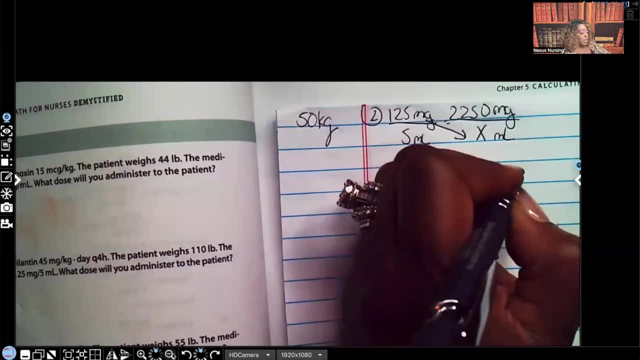 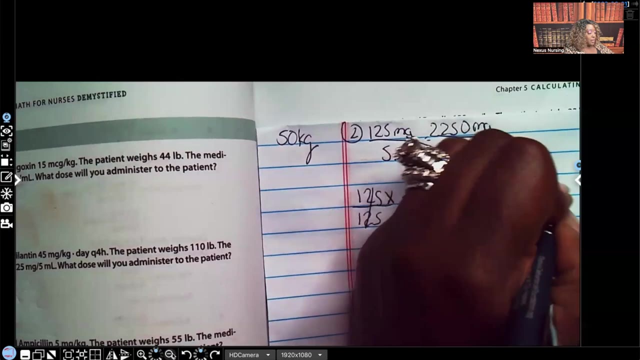 250.. How many times? let's plug that in 11, 250.. Divided by 125, 90. It goes 90 times. So that means I'm going to be giving 90 MLs per day. How do I know it's ML? Remember, I'm solving for X. X is ML, So that's how I know. 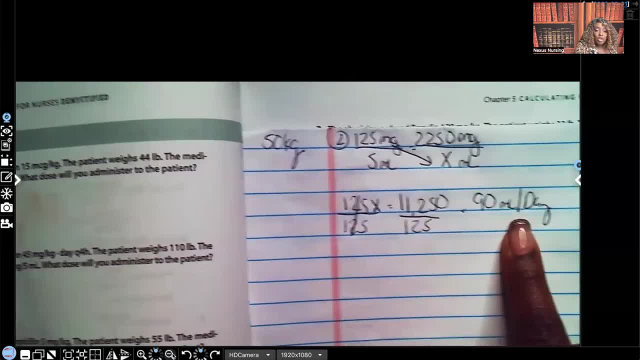 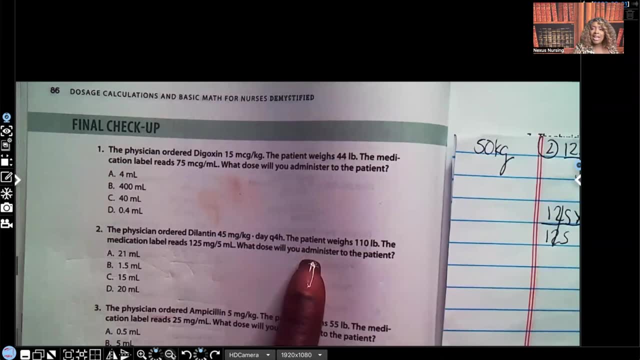 that's my unit, So I'm giving 90 MLs per day. but I want you to go back to the question. Look what it says: What dose will you administer the patient? Now, how much you're going to give per day. What dose will you administer the patient? What dose will you administer the patient? 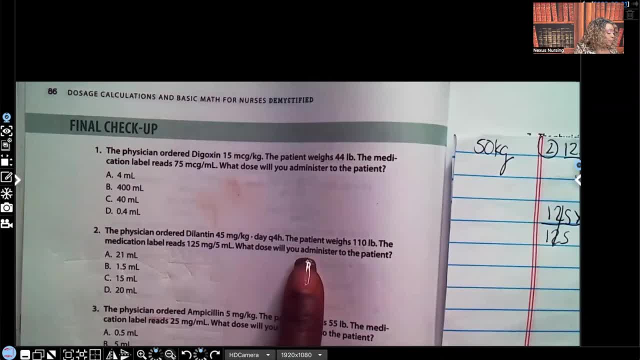 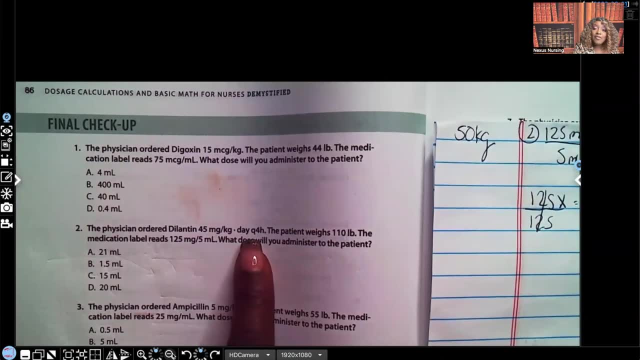 What dose? So if you go back to the order and it says that we're giving this medication every four hours, if you're giving a medication every four hours, how many times are you going to be giving that medication? Six, Why Four times six is 24.. Just like if it said to give. 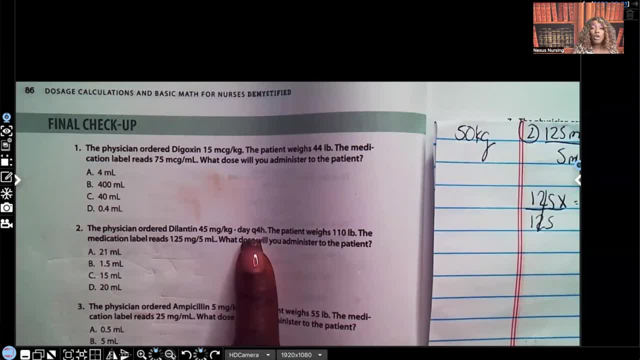 the medication every six hours, then you know you'd be giving four doses. But since it said to give every four hours, we know that we're giving six doses. We are giving this medication six times. Why is that important If we're giving 90 milliliters per? 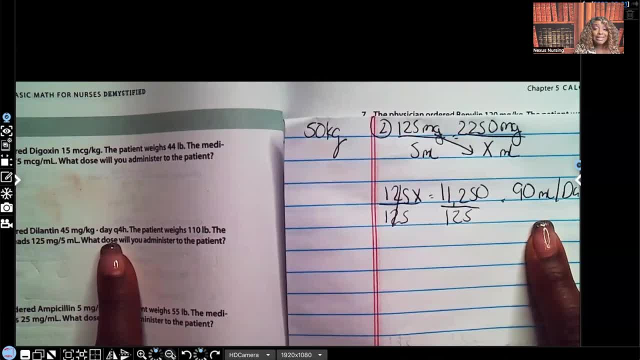 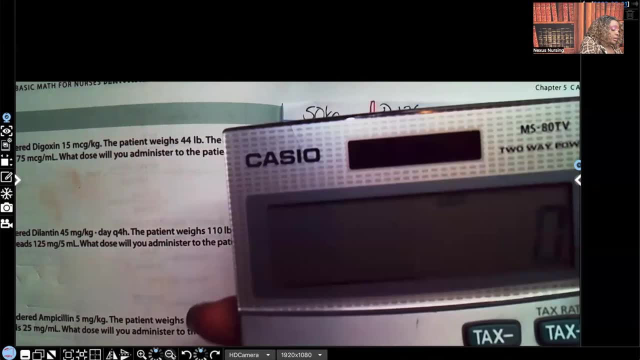 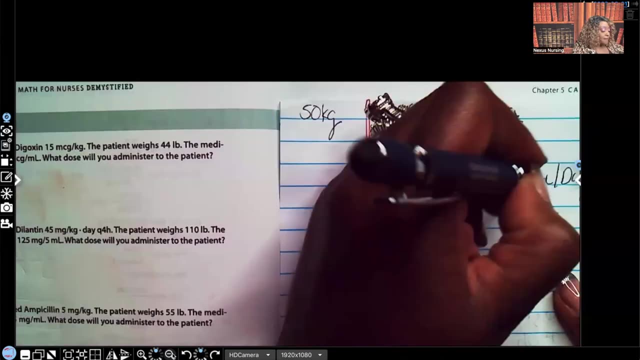 day, but we know we're giving this medication six times. we have to divide that 90 by six to get our real answer. So let's do it: 90 divided by six, 15. We're going to be giving 15 MLs per dose. 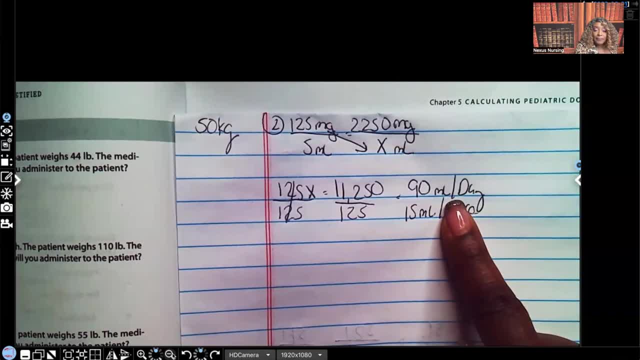 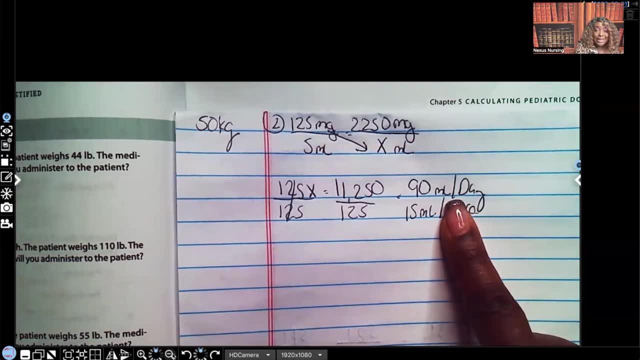 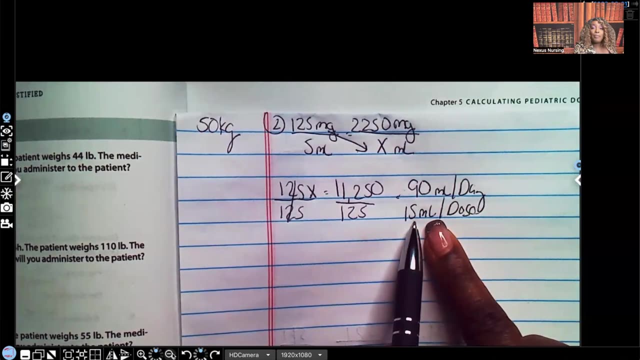 So, even though we're giving 90 milliliters a day because we're giving this medication every four hours, we know that means we have to give this medication six times a day. We're taking this total dose of 90 and we're dividing it by six And that's how we get the 15 MLs per dose Be very. 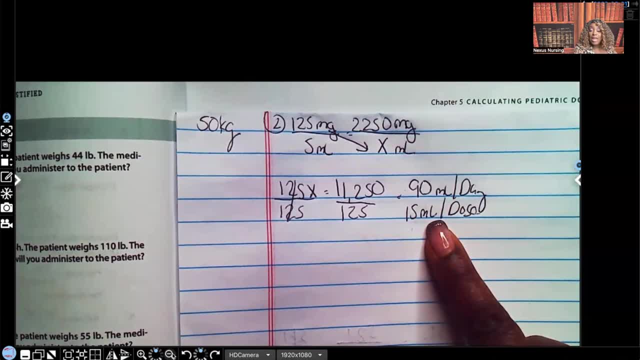 careful, because that's how the test writers will try to trick you. It might ask you per day and it might ask you per dose. per day is always going to be the total, the accumulation of what you're going to get for that entire 20.. 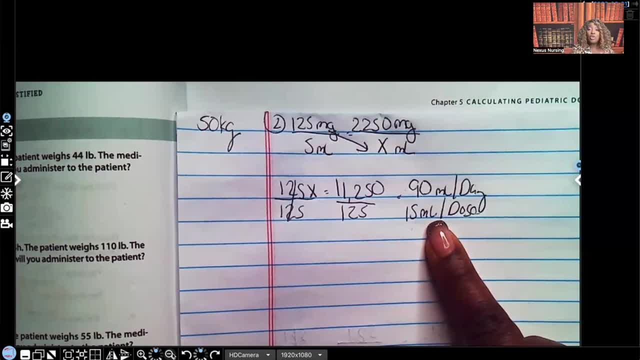 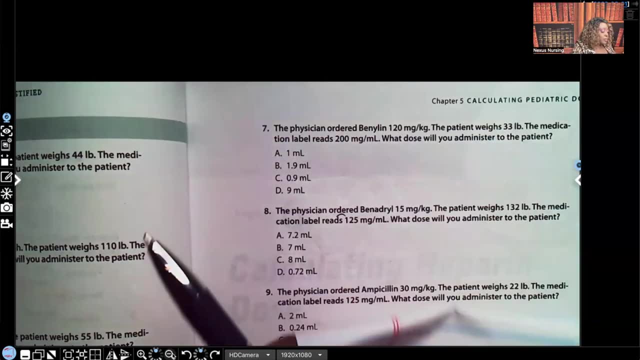 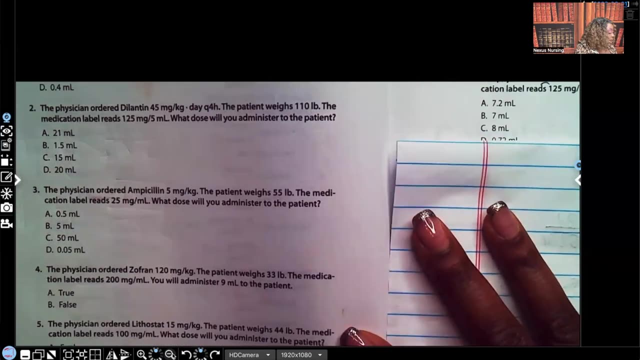 24 hours versus the dose, which is how much you're going to give every time you give that particular medication. All right, let's move on to number three. Look at number three. Number three says the physician ordered ampicillin five milligrams per kilogram and the patient 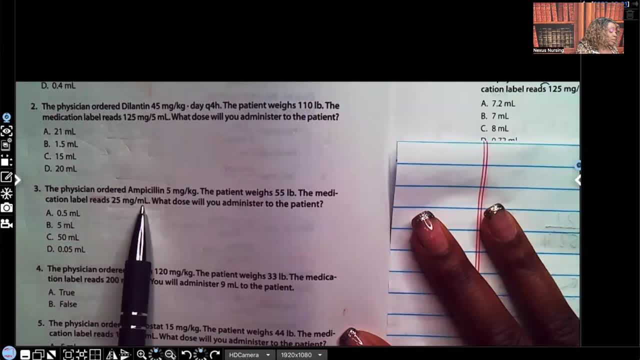 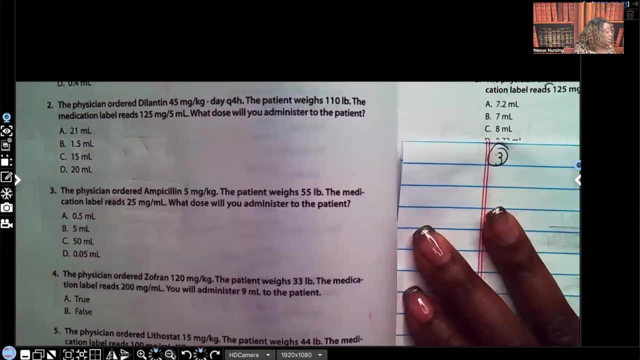 weighs 55 pounds. The medication label reads 25 milligrams per milliliter. What dose will you administer to the patient? What dose will you administer to the patient? What dose will you administer to the patient? Again, let me write my number three. This is number three. we're doing Again. we're. 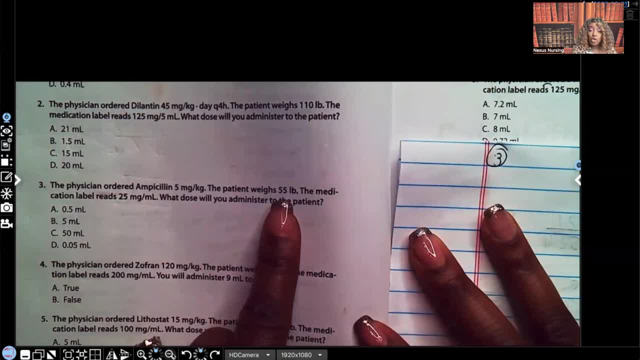 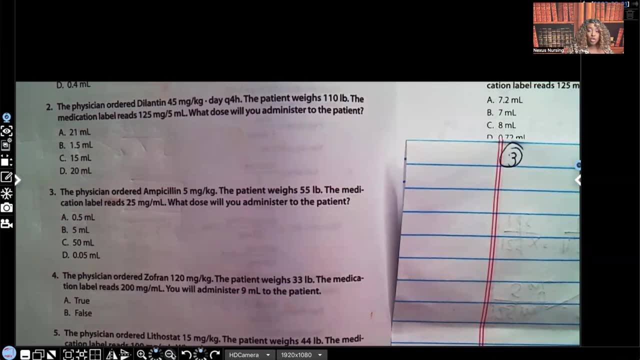 going to convert our pounds to kilogram. That's the first thing we're going to do. So we're going to do 55 divided by 2.2. And you should get 25.. Okay, So let's write it here on the side, so we 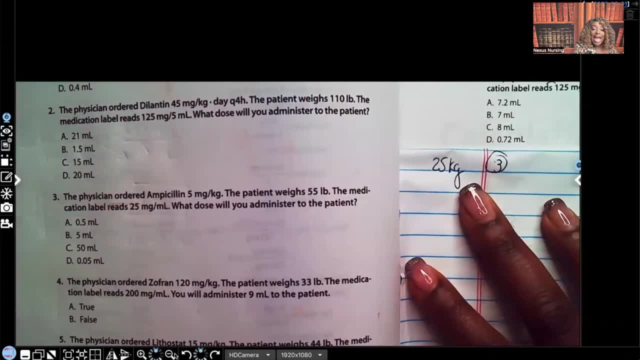 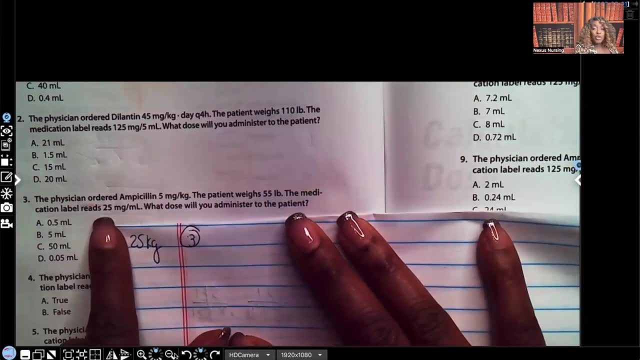 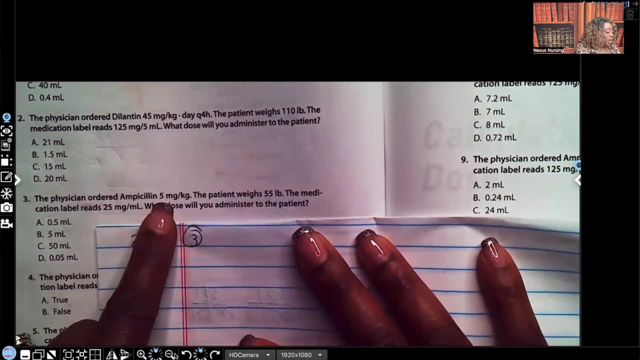 don't forget, Our kid weighs 25 kilograms. Now that we know how many kilograms our child weighs, we can do the math. As I said, always start with your label, Always start with what you have. What you have is not going to change If you take a look. look at what the doctor wants- five milligrams- And what we. 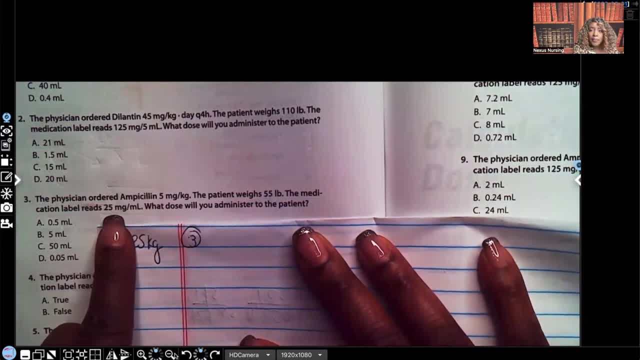 have is 25 milligrams, So wonderful, We don't have to convert. But let's say you do have to convert. What you have on hand is what you have on hand. You're not going to convert what you have on hand. You're going to convert what they want to what you have on hand. So let's go ahead and 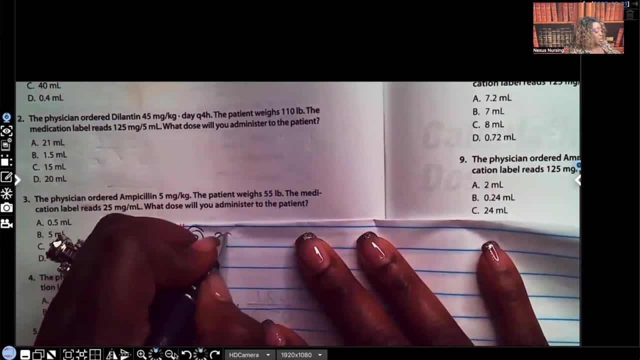 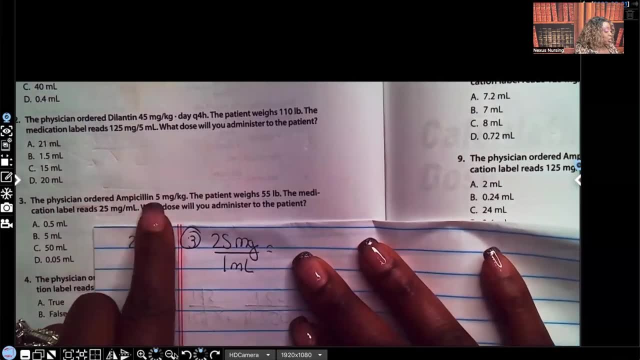 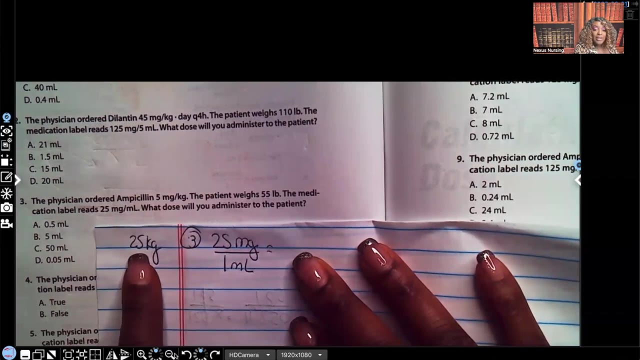 write down 25 milligrams per one ml. 25 milligrams To one ml Equals again. now we go to what's ordered, which is five milligrams per kilogram, And all we're going to do is multiply that five milligrams times our 25 kilograms to see what. 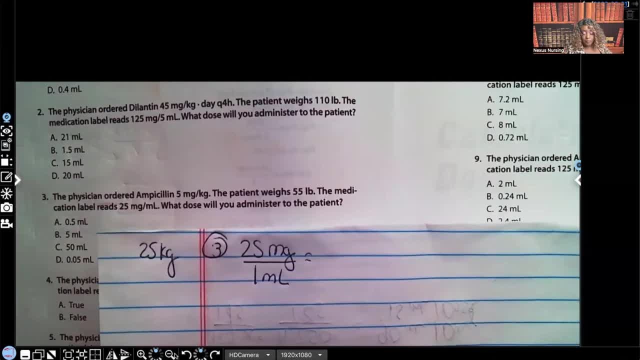 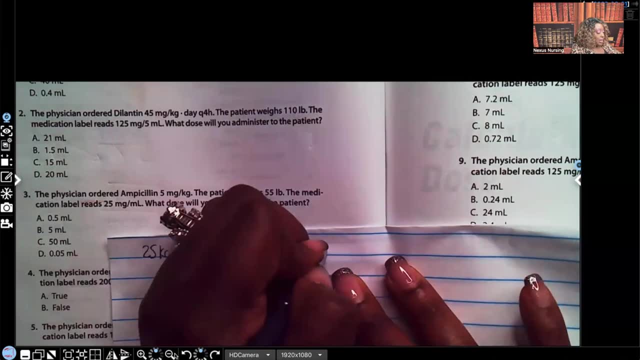 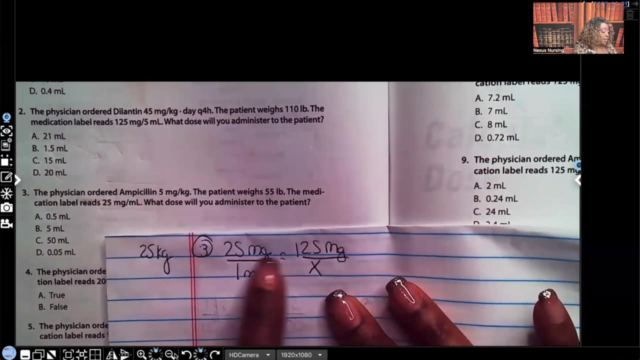 we're going to do Five times 25.. And you should come up with 125.. 125 milligrams over what X. X is what you're solving for Milligram, Milligram, Milliliters. X is going to be what Milliliters, Whatever you're solving for. 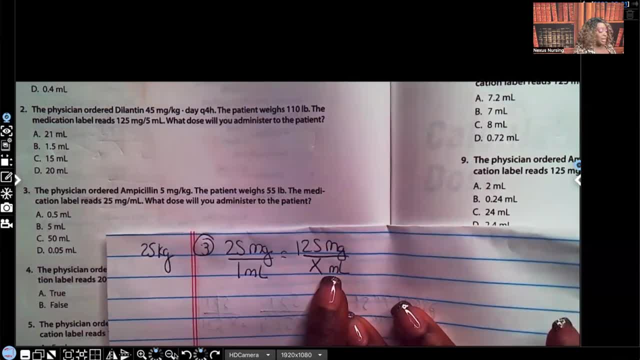 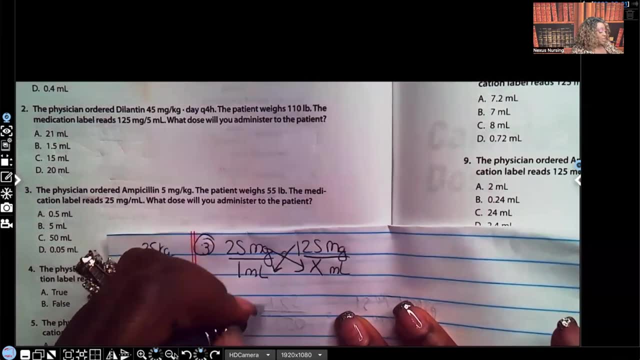 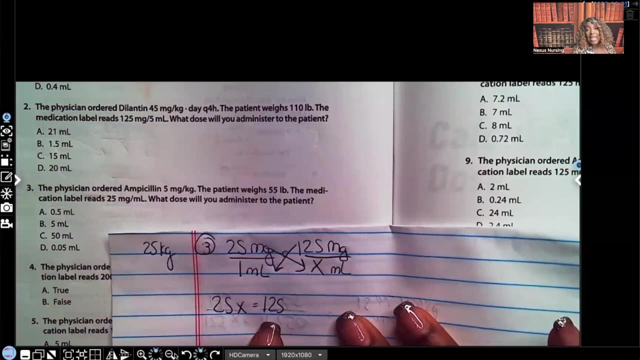 is going to be ml. We set up our problem. Now we cross: multiply. 25 times X equals 25X. 125 times 1 equals 125.. Now I have 25X equals 125. We have to get X by itself. What are we going to do? We're. 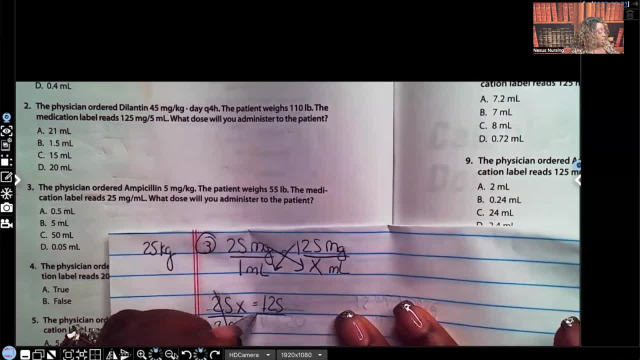 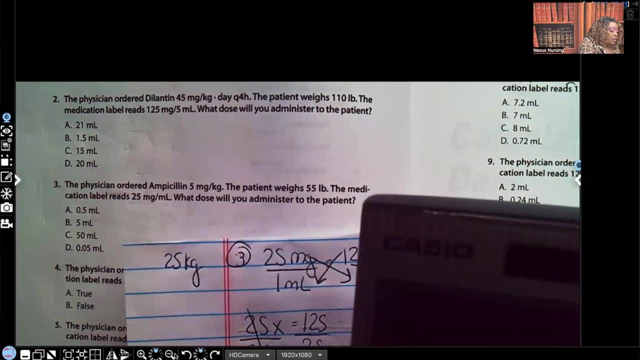 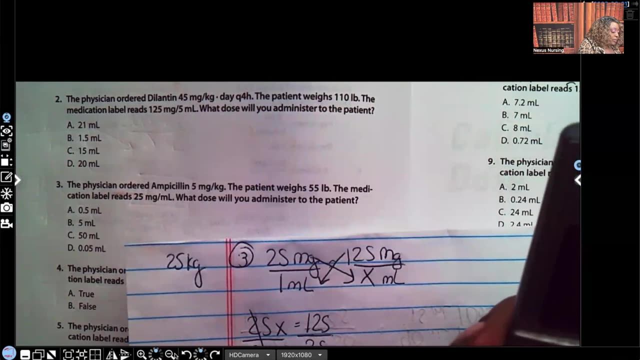 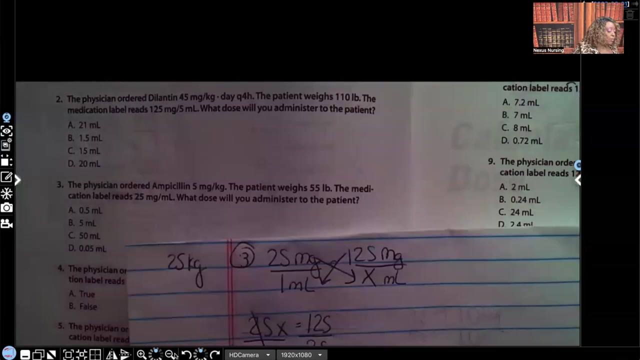 going to divide by both sides, 25.. 25.. 25 goes into 125.. How many times? Five times. Just plug it in: 125 divided by five. Why do I have 25?? That's not right. 125 divided by 25.. Just joking, There you go. Five, Right, So my? 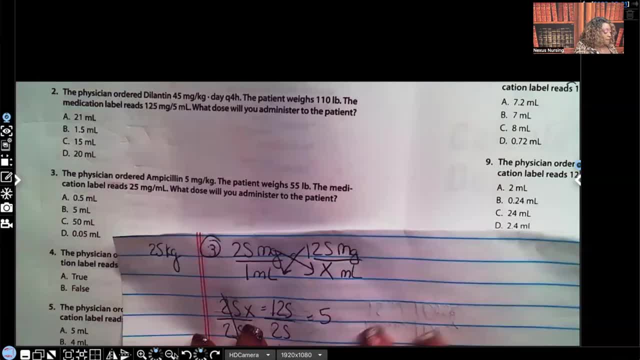 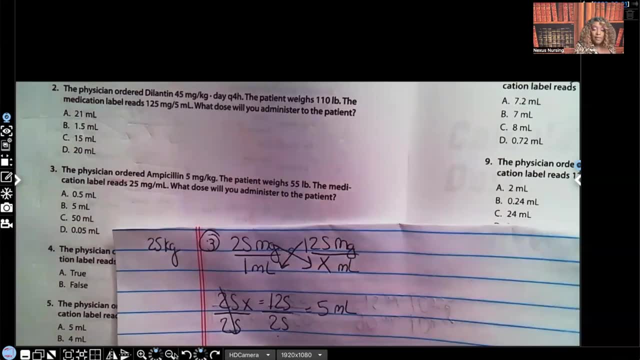 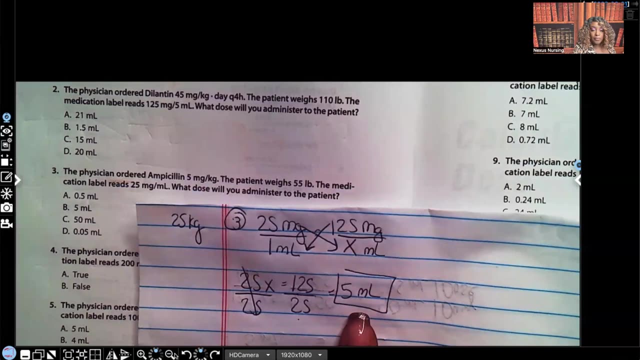 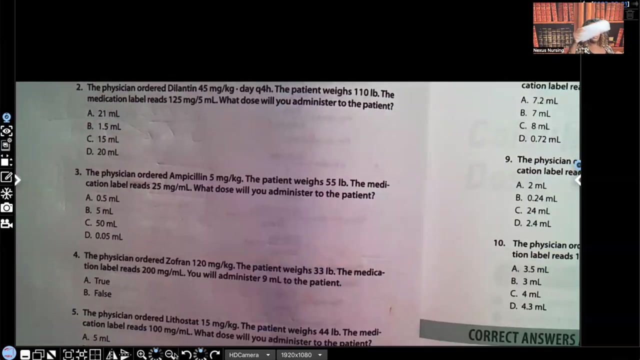 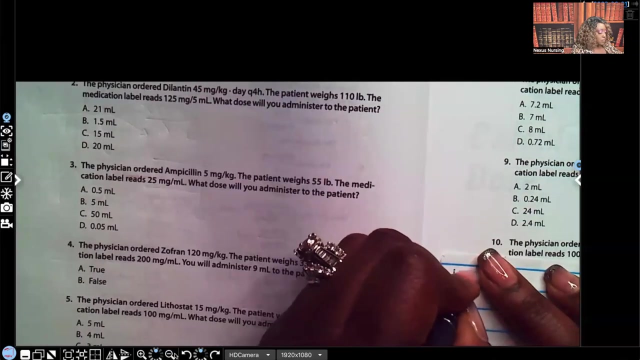 answer is five, Five. what We're solving for X? Five Five mls. Let me make sure I'm right. Number three: Yep, There you go, Five mls. Okay, Let's do number four, Number four. Look at the question. 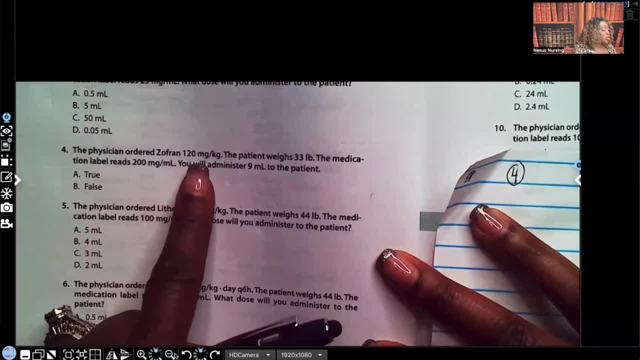 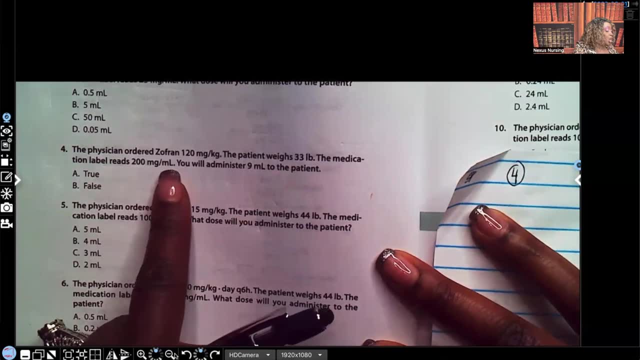 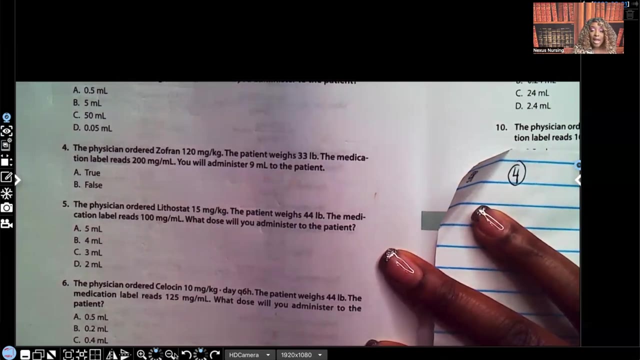 It says the physician ordered Zofran 120 milligrams per kilogram. Patient weighs 33 pounds. The medication label reads 200 milligrams per ml. You will administer nine mls to the patient. True or false? I have no idea. Let's do this math and figure it out. What is the first thing we're 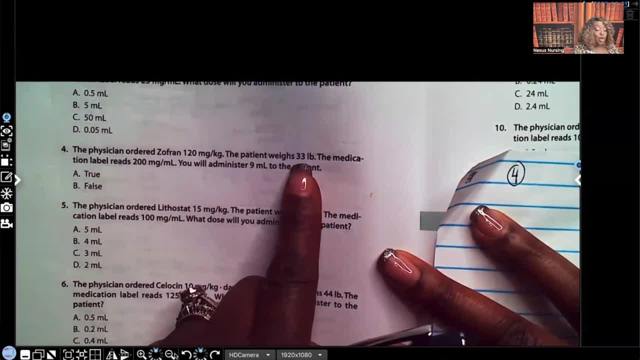 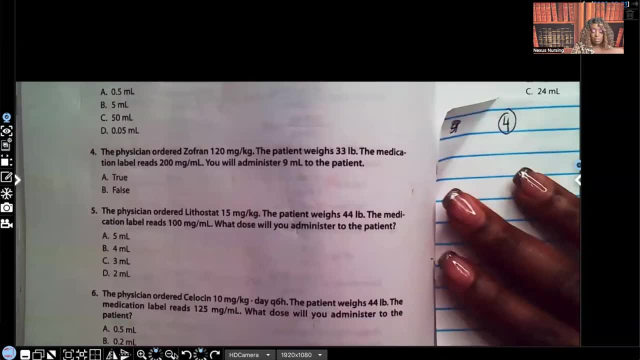 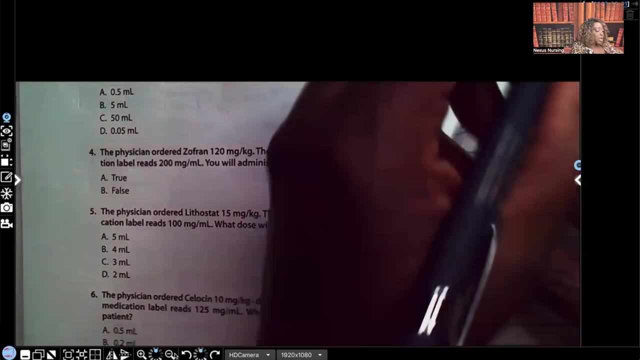 going to do? We're going to turn that pound into kilograms, So that 33 pounds do 33 divided by 2.2.. Oh, And that gives you 15.. So we know our kid weighs 15 kilograms. Now that we know the kid weighs 15, 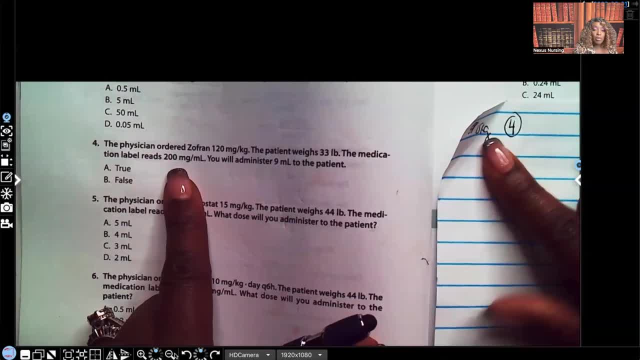 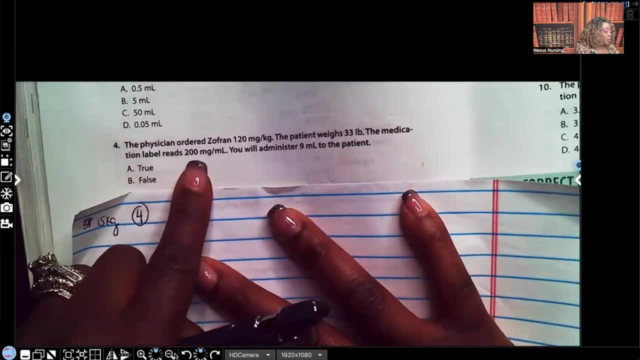 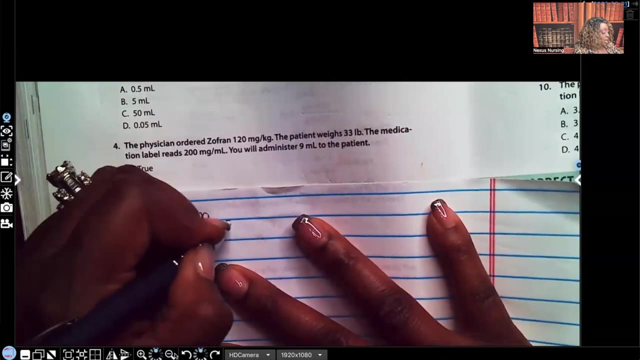 kilograms. let's start our math Again. always start with what you already have. Let me move this down here under number four so you can see better. Always start with what you have, which is 200 milligrams per ml. So I'm going to write 200 milligrams over one ml is equal to: 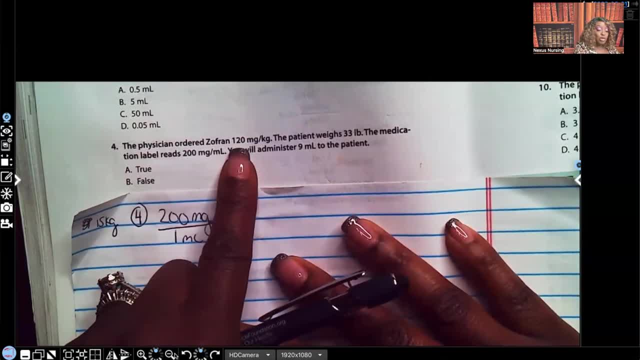 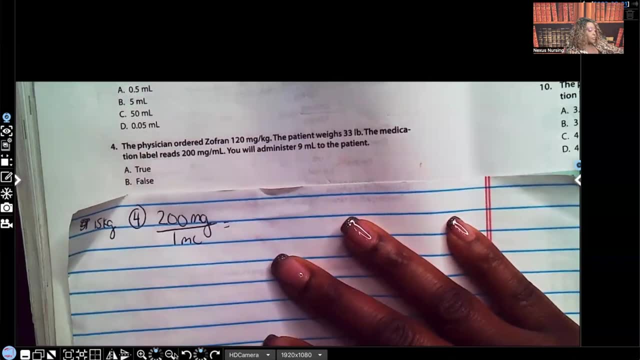 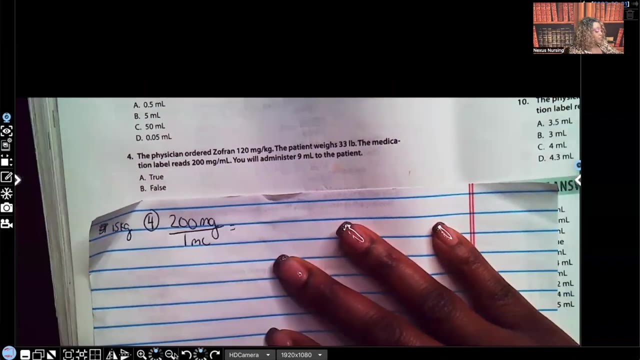 now look at what's ordered: 120 milligrams per kilogram. So we're going to multiply that 120 times our kilogram, 120 times 15.. 120 times 15, that gives you 1800.. So we're going to give 1800 milligrams over X. We're not done. 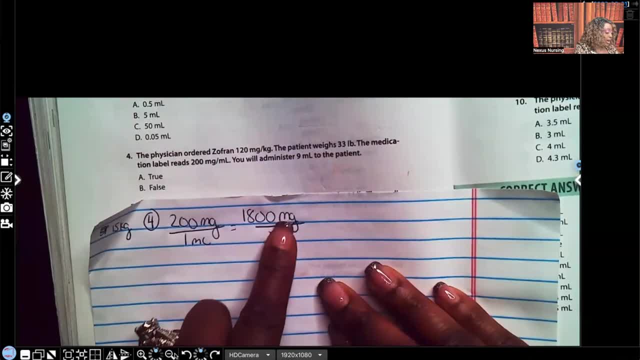 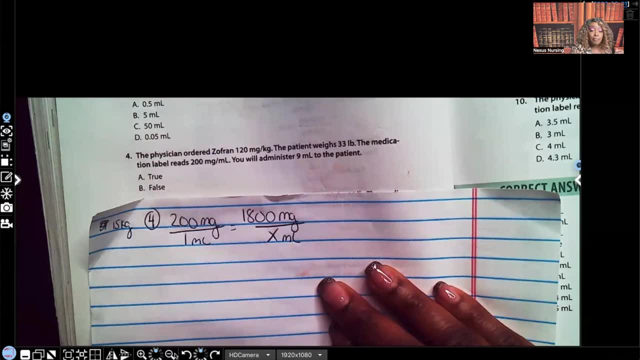 We have to put a unit on the X. You see, milligram, milligram, milliliter, We're going to X Milliliters. Whatever we solve for is going to be an ml. Now that our problem's set up. 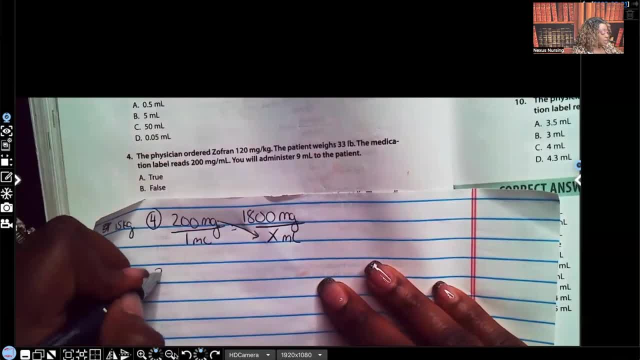 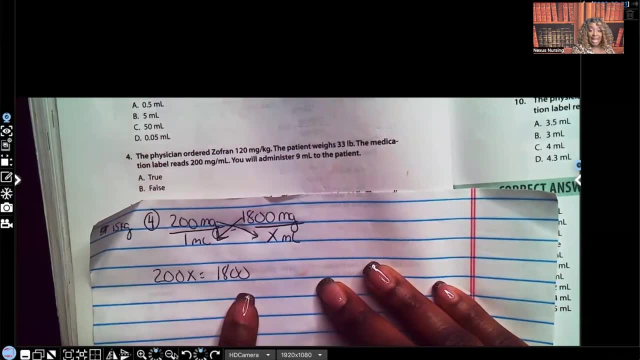 let's cross. multiply 200 times X is going to be 200 X. 1800 times one is going to be 1800.. 200 X equals 1800.. We have to get X by itself. So what are we going to do? Divide by both sides. 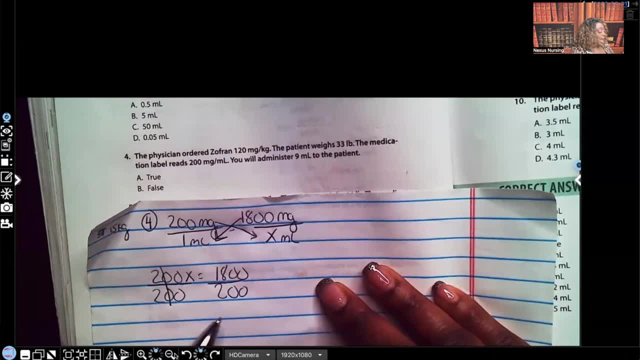 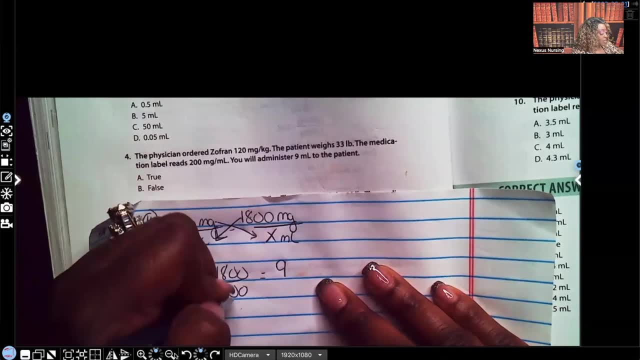 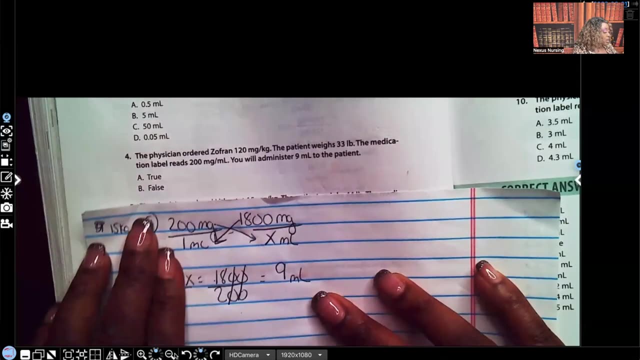 200, 200.. How many times did 200 go into 18? Two goes into 18 nine times. Let me get rid of this, So it's nine. But remember we have to have our unit nine mls, So saying we're going to give nine ml, Is this true? Yes, 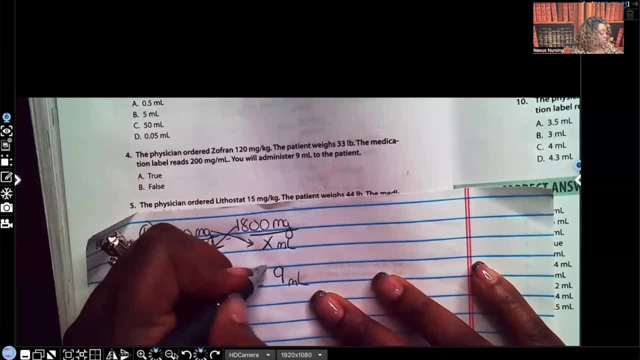 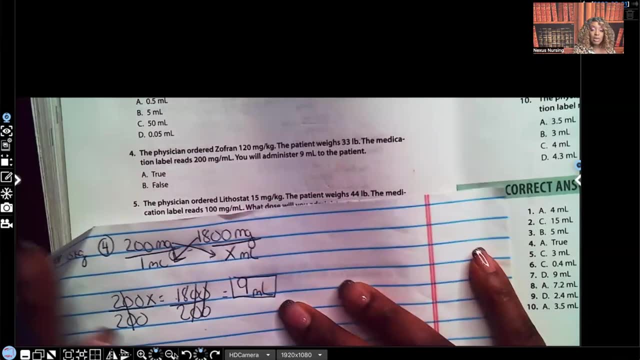 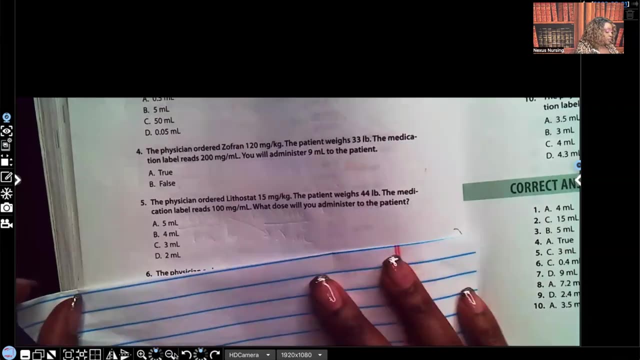 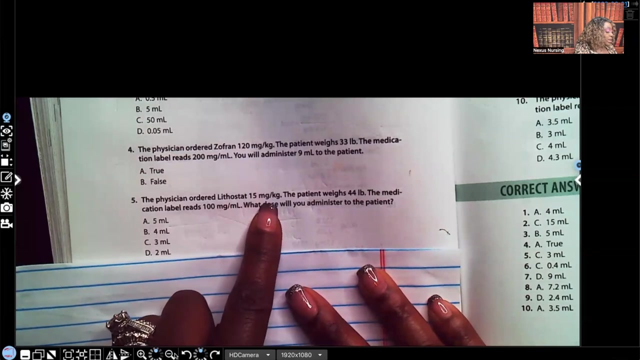 it's true. That's exactly what we're going to give. Let's check the answer. Number four: Yep, true, That's what we're giving. Let's do number five. It says the physician ordered lithostat 15 milligrams per kilogram. Patient weighs 44 pounds. 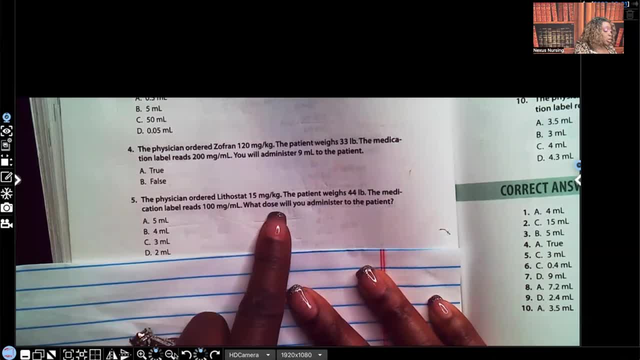 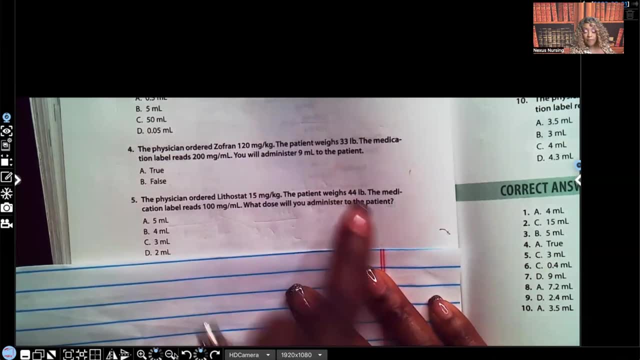 The label reads 100 milligrams per milliliter. What dose will you administer to the patient? As always, we're going to start with our pounds. Convert that to kilogram 44 divided by 2.2. 20.. So our kid weighs 20 kilograms. What number are we on? 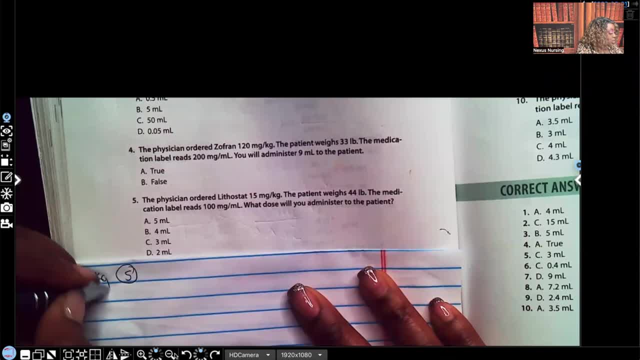 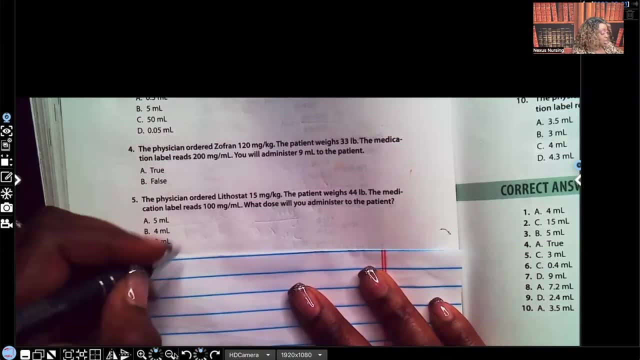 We're on number five. Okay, so I'm going to write my 20 kilograms here, So I don't forget. What are we going to do next? We're going to start with what we have. We're going to look at the label. It says 100 milligrams per ml. Drop that down. 100 milligrams per one ml is equal to: 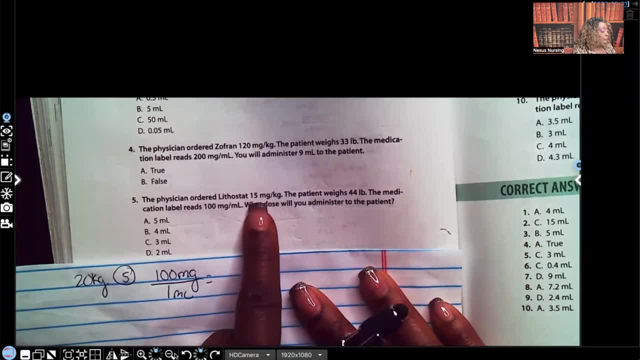 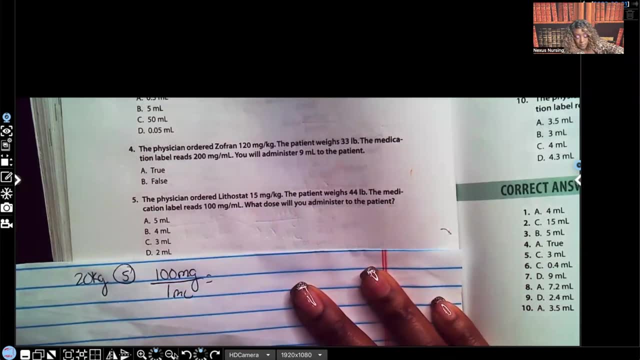 remember up here what's being ordered: 15 milligrams per kilogram. Multiply that 15 times your kilogram, 15 times 20.. And that gives you 300.. Why do I feel like we did this already, But maybe not? That gives me 300.. 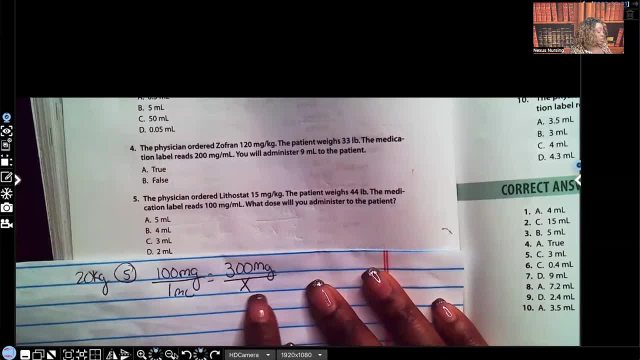 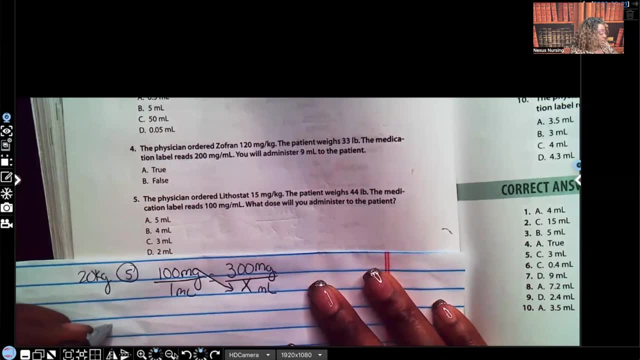 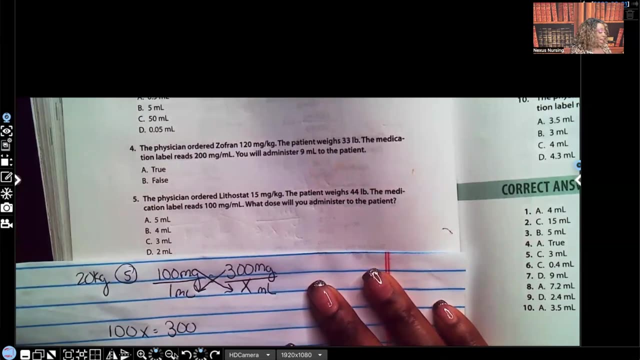 300 milligrams over x. What's my unit going to be? ml? What do I do next? I cross multiply: 100 times x equals 100 x, and then 300 times 1 equals 300. now i have 100 x equals 300. let me put this over. 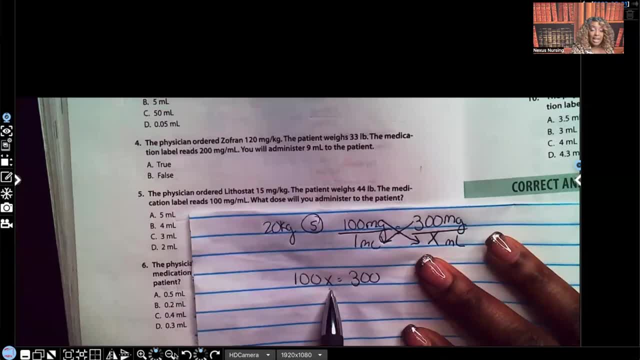 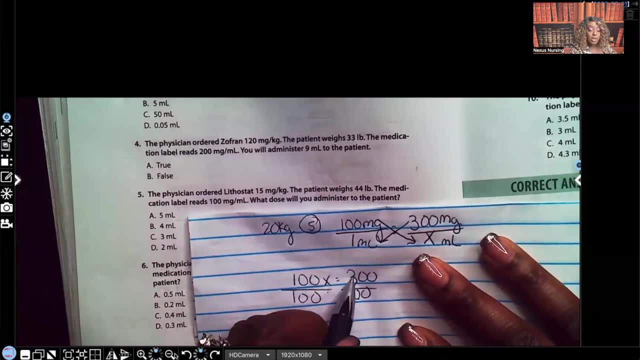 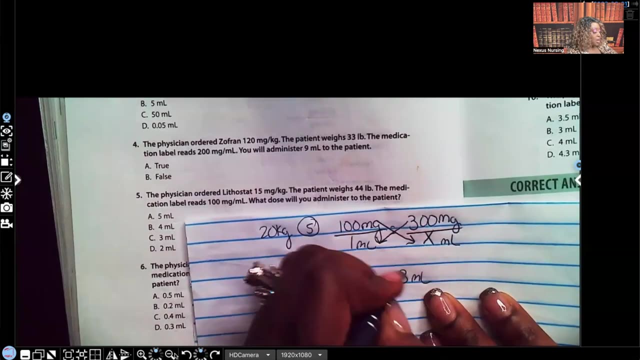 here, so you can still see i got to get x by itself. so i'm going to divide by both sides: divide by 100, divide by 100, 100 goes into 300. three times three. what ml? always go to x to see what your unit is. if you forgot, we're giving three mls. that's for number five. three ml, right here. 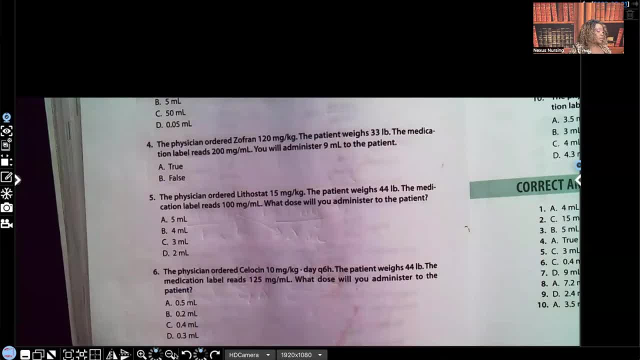 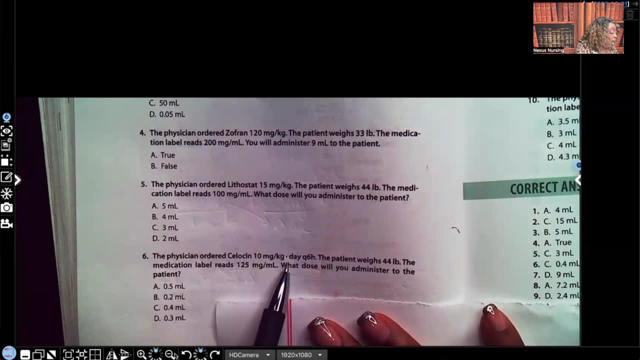 all right, let's do number six for number six. it says: the physician ordered cellosin 10 milligrams per kilogram uh per day, every six hours. the patient weighs 44 pounds. the label reads 125 milligrams per ml. what dose will you administer to the patient? nothing changes. we're going to do the same. 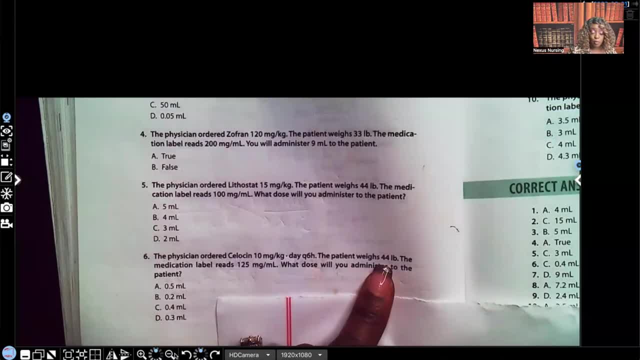 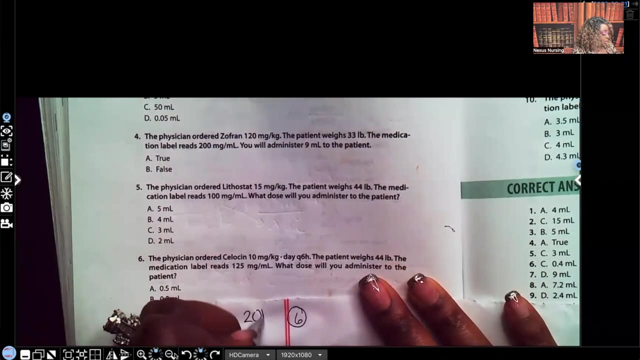 thing. we're going to start with our pounds and convert that to kilograms. so let's do 44 divided by 2.2, that gives us 20. our kid weighs 20 kilograms. 20 kilograms, all right. next we're going to look at what we have, which is our label. it's 125. 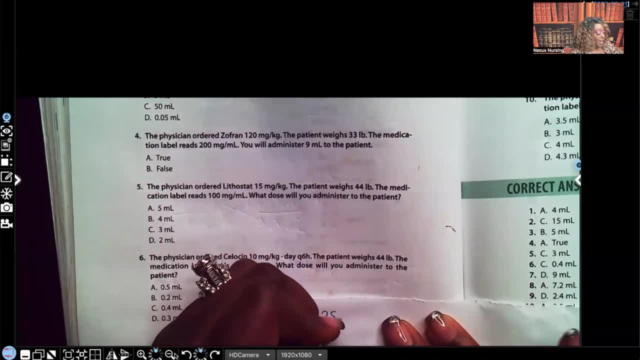 per 1 ml. let's write it down: 125 milligrams per 1 ml, and that equals- let's see what's- 129 milligrams per ml. all right, so let's do 44 divided by 2.2, that gives us 20. our kid weighs 20 kilograms. that gives us 20 kilograms. 20 kilograms, 20 kilograms. 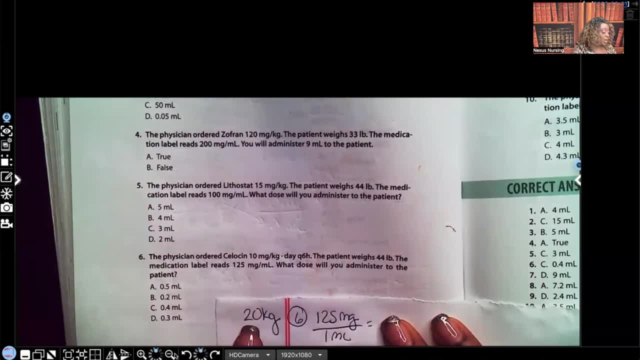 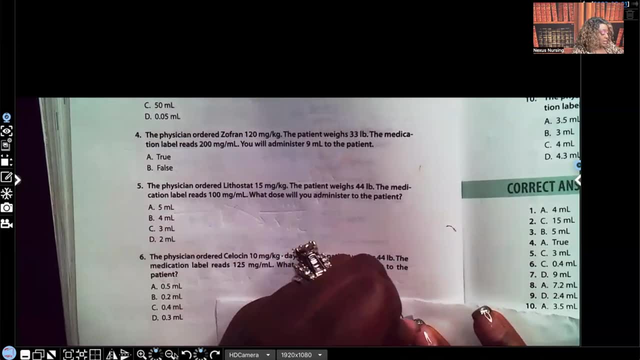 Let's go to what's ordered: 10 milligrams per kilogram, and our kid weighs 20 kilograms. So you're going to do 10 times 20.. What does that give you? Two at my zeros, That gives you 200 over X. 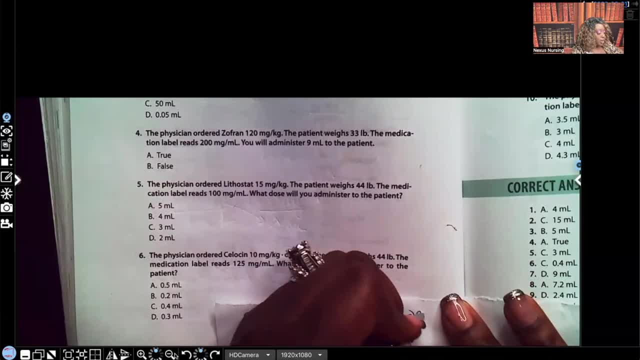 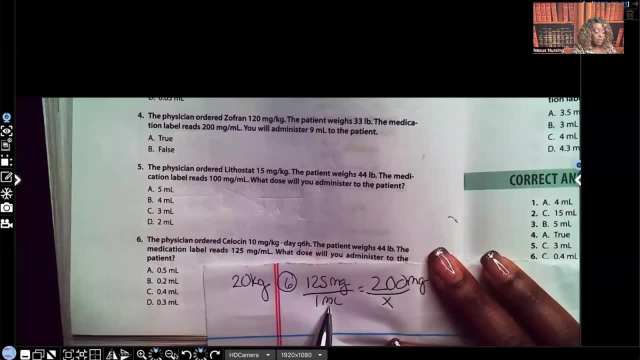 Remember, we have to have our units. This is milligram, So this over here has to be milligram, and this is milliliters. Move this up for you: This is milliliters, so this has to be milliliters. 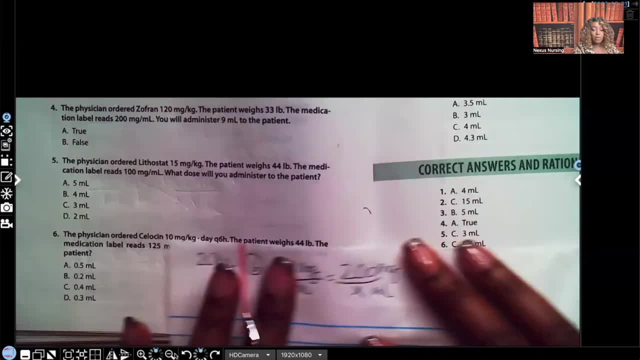 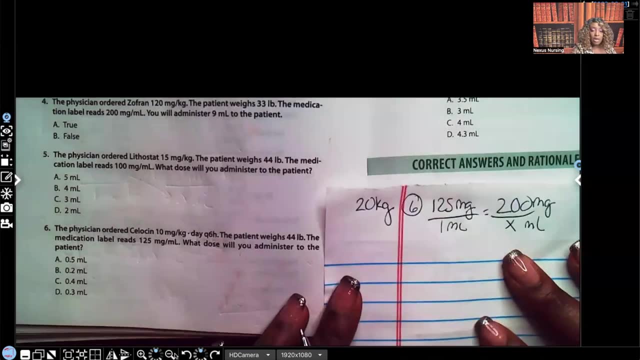 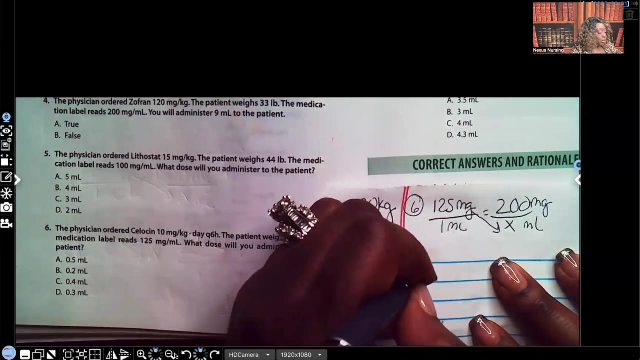 Okay, great, Let me move here so you can see the math. I want you to still be able to see what I'm doing. Okay, you can see this. Now that this is set up, we can cross: multiply: 125 times X equals 125X, and then 200 times 1 is equal to 200. 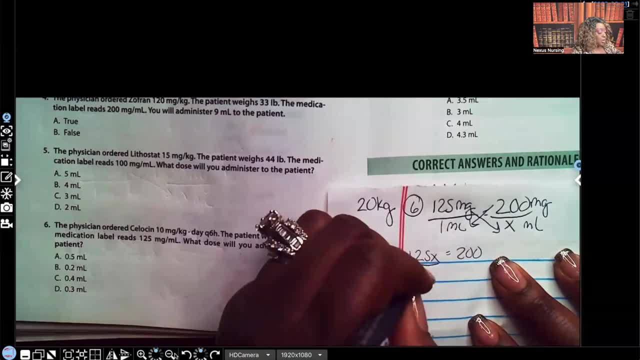 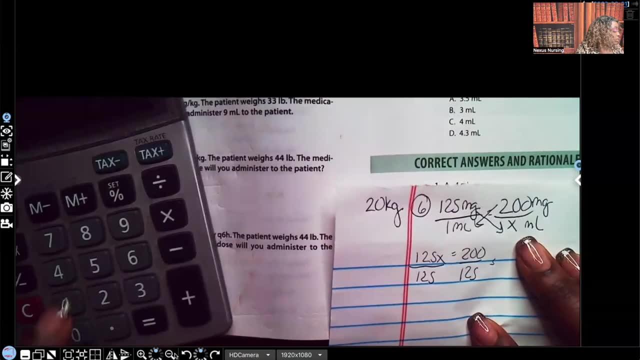 125X equals 200.. We got to get X by itself, so we're going to divide by 125.. 125, how many times is 125 going to 200? 1.6.. Number 6, am I right? 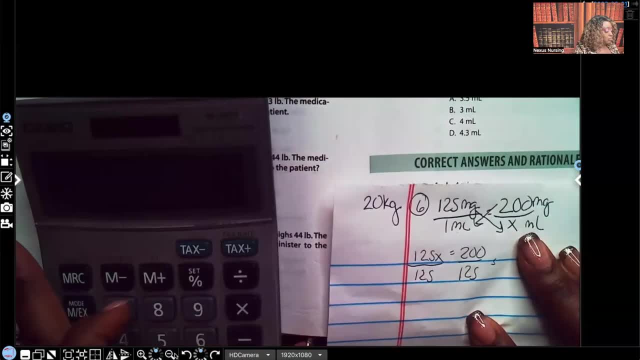 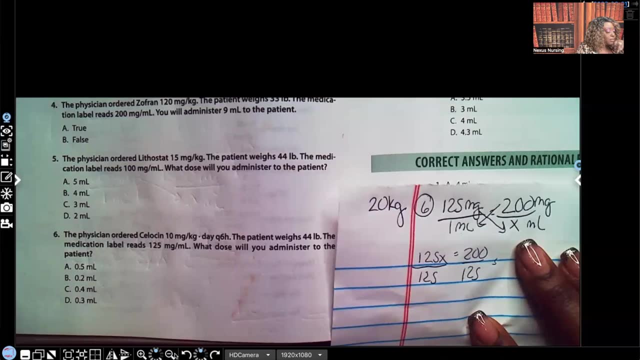 Nope, I'm all off. I did something wrong. Let me see if I can figure out what I did wrong. Number 6, the answer is supposed to be 0.4.. Okay, let's see what I did wrong. Okay, let's see what I did wrong. 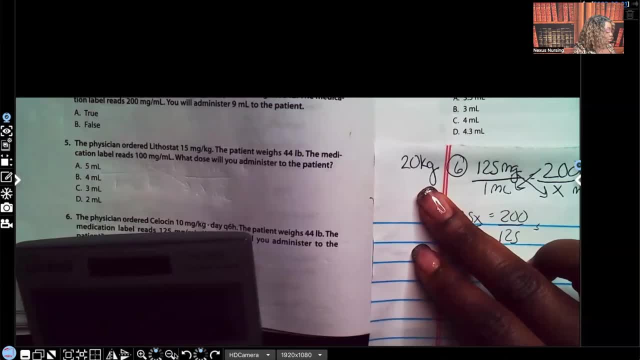 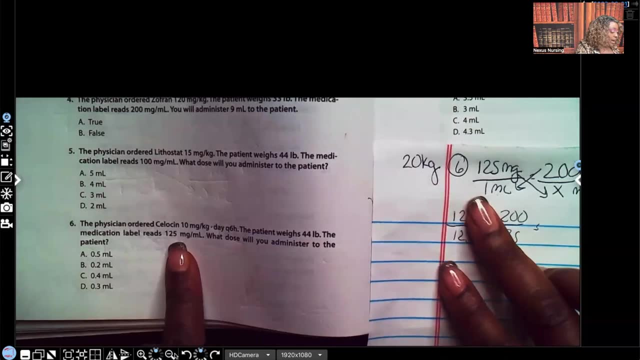 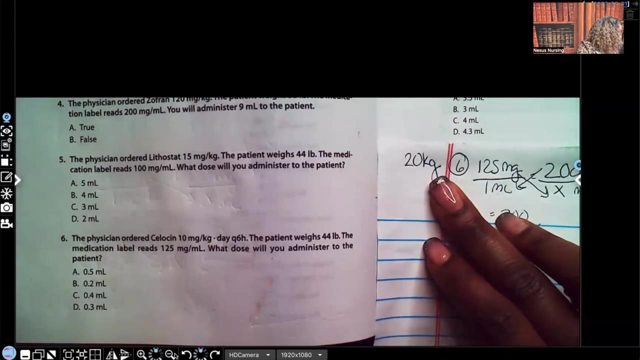 My kid weighs 20 kilograms. I'm going to do 44 divided by 2.2.. Okay, so that's correct. Then I do: 125 over 1 ml is equal to 10 times 20, 200,. yep, 200 over X. 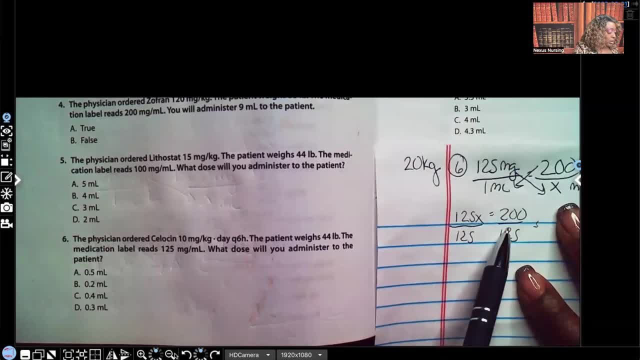 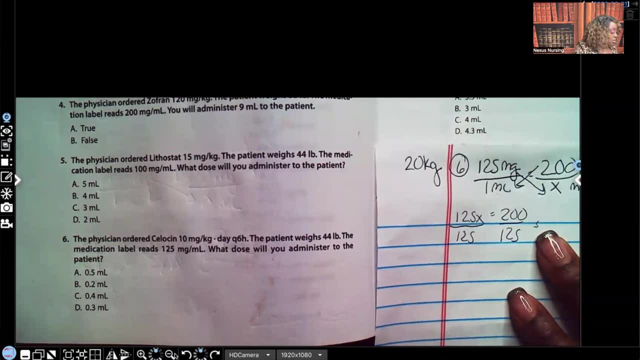 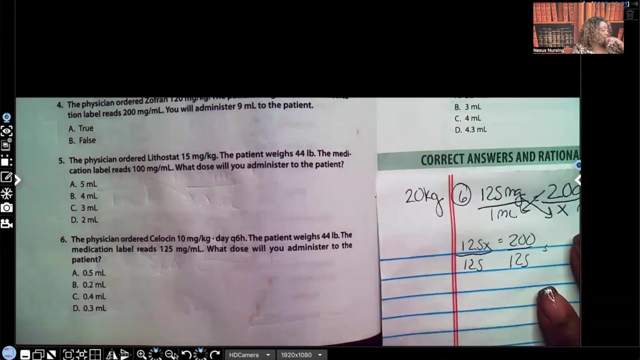 Then I cross multiply. 125X is equal to 200.. What am I doing wrong? 200 divided by 125, wait, 125 divided by 200.. I don't know what I did wrong. I'm going to start over again. 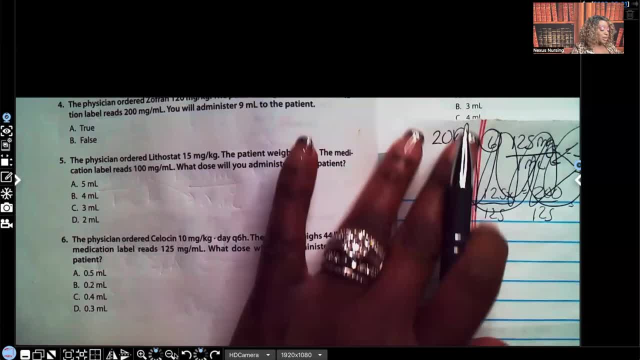 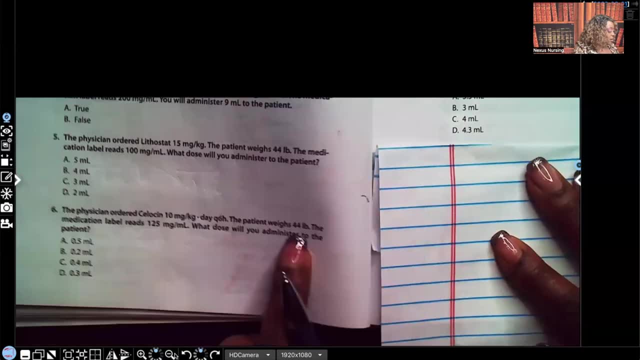 If you guys see where I went wrong, let me know in the comment section, because I'm starting this all over again. I'm trying to figure out where I went wrong. Let's start over Pounds 44 divided by 2.2.. 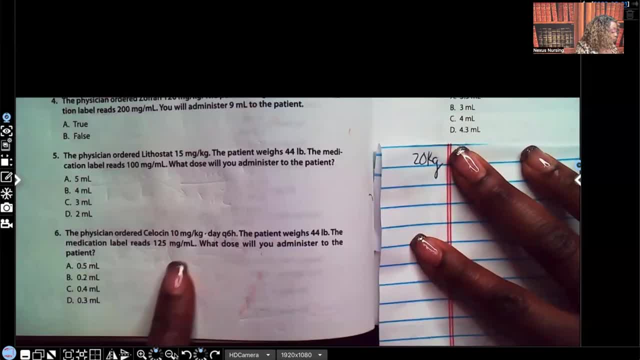 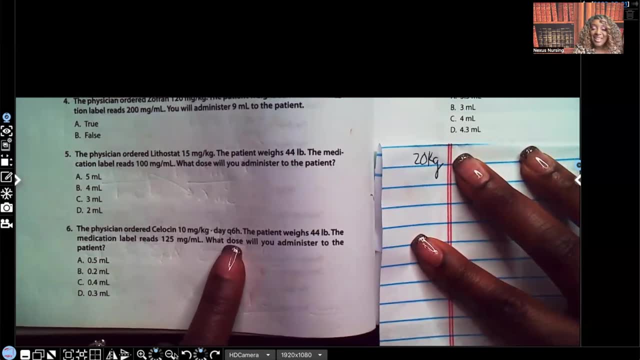 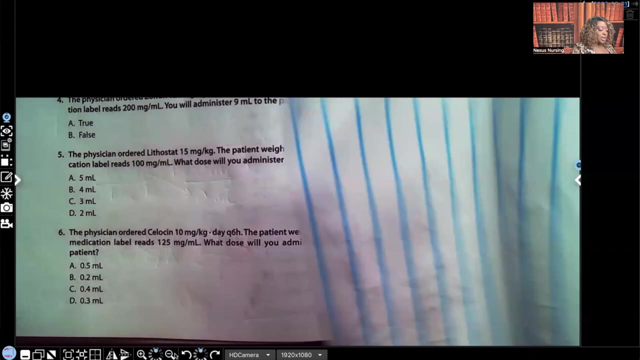 Kid weighs 20 kilograms. I'm going to put that over here. I know what I did wrong. Guys, look What dose will you administer? I did the math right. Take a look Where's that math I was doing Okay. 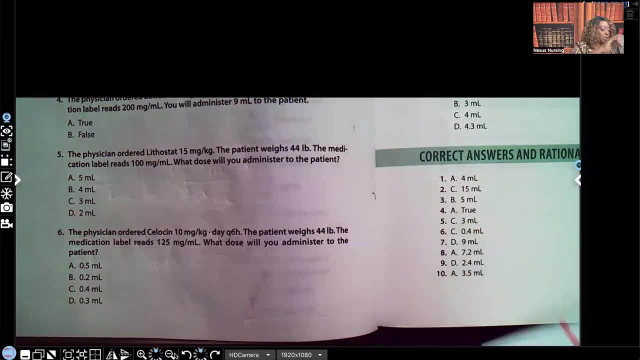 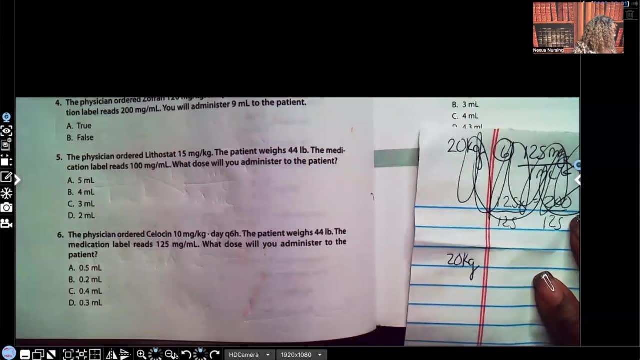 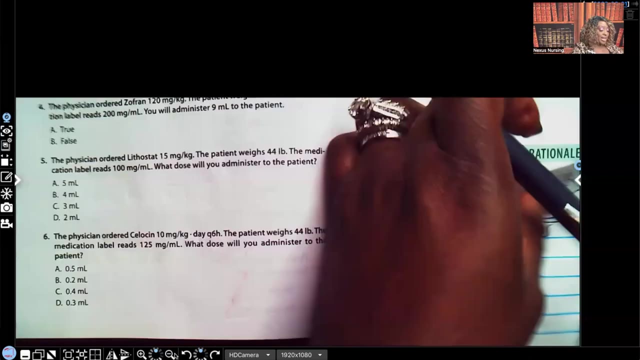 Oh, I'm annoyed with myself. Here it is, So wait a minute. When I did 200 divided by 125, my answer was 1.6, but that's for the day. 1.6 ml, this is for the day. 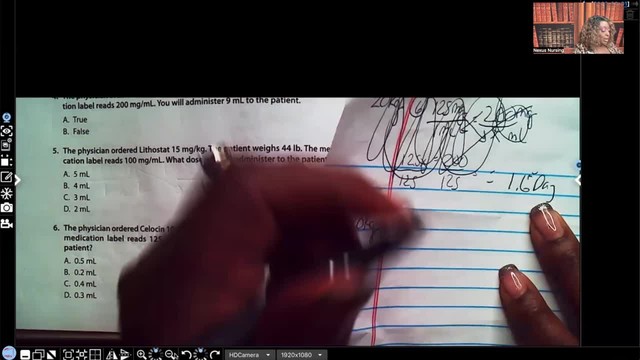 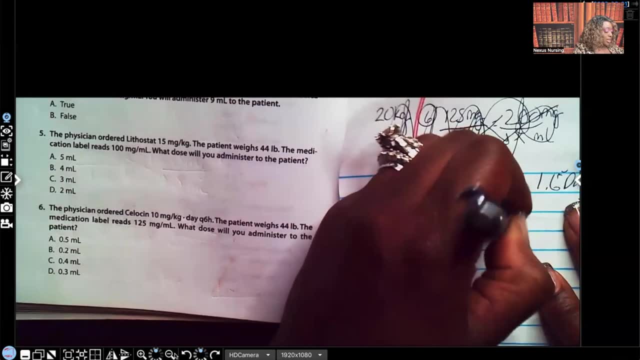 The question's asking me dose, So let me do the dose and see if I was right all along. So if I'm giving 1.6.. 1.6 ml for the entire day and it says that I'm giving this medication every six hours, 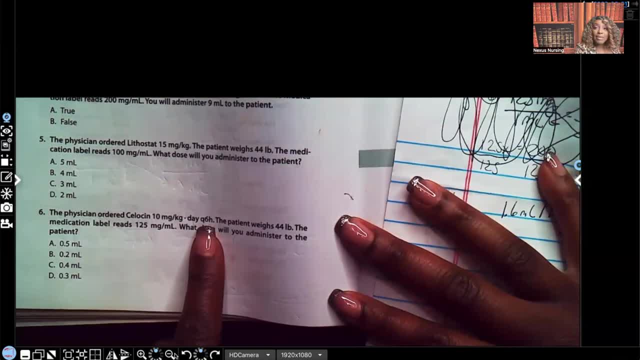 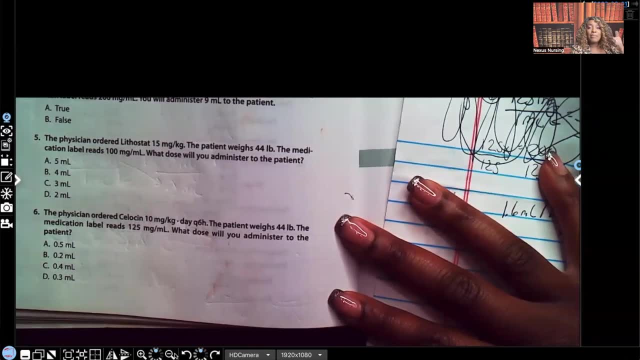 If I'm giving this medication every six hours, that means I'm giving this medication four times a day. Why? Because six times four equals 24.. If I'm giving this medication every six hours, that means four times a day I'm giving this medication. 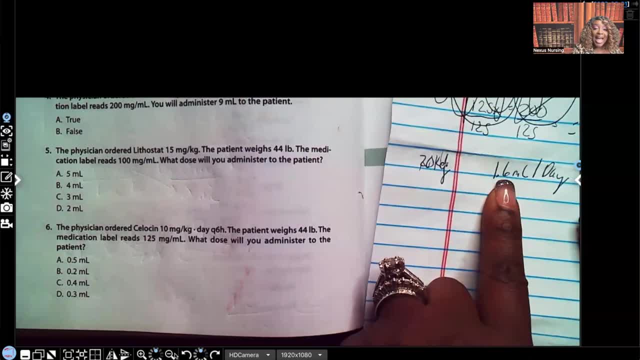 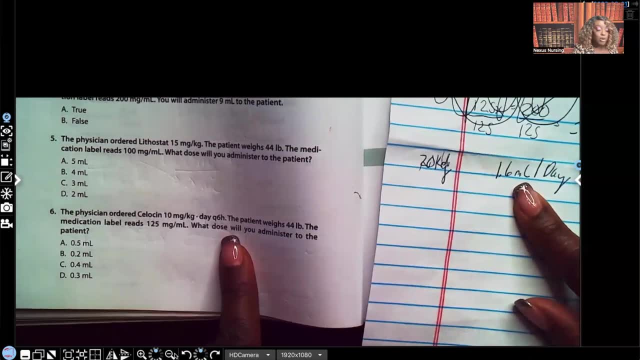 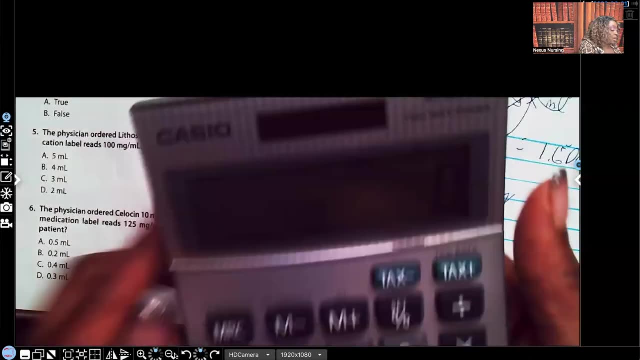 That means this answer of 1.6 that I got. I have to divide that by four, Because I'm giving it four times 1.6 divided by four, and this better be the right answer: 1.6 divided by four: 0.4.. 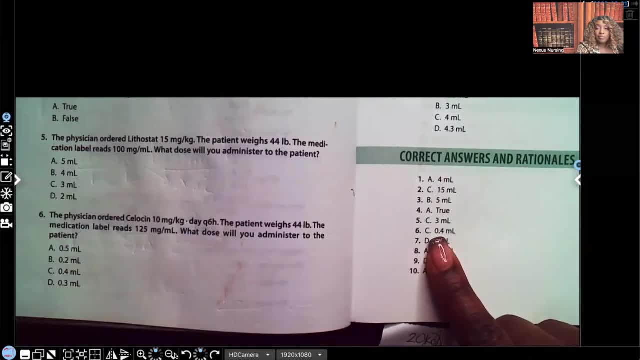 That is the correct answer: 0.4.. You see what I did- And I've been doing this for years- and I made that simple mistake- Don't do it. And I just warned you guys about it. and I did exactly what I warned you guys not to do. 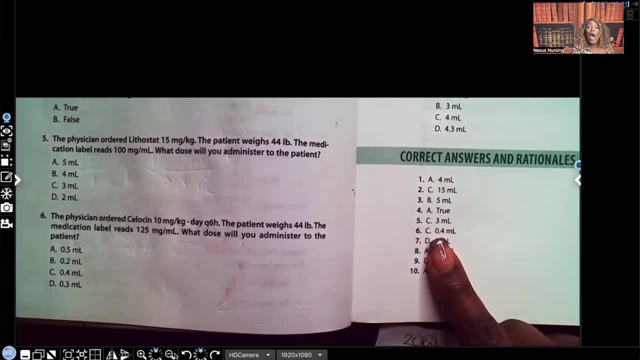 Okay. So, with that being said, always go back and check After you figure out how much you're going to give that patient per day. make sure if it's per dose you have to divide what you're giving per day So you don't mess up on your math. 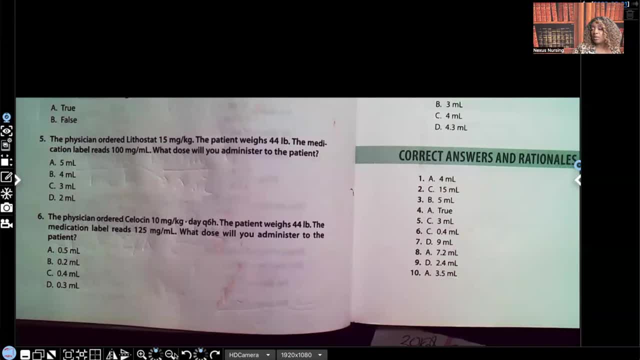 It's so funny, guys. I really squeezed in this medication. I squeezed in this video. I have to go to the Geek Squad and get one of my laptops fixed. My appointment is up so I have to run, But I'm going to continue. 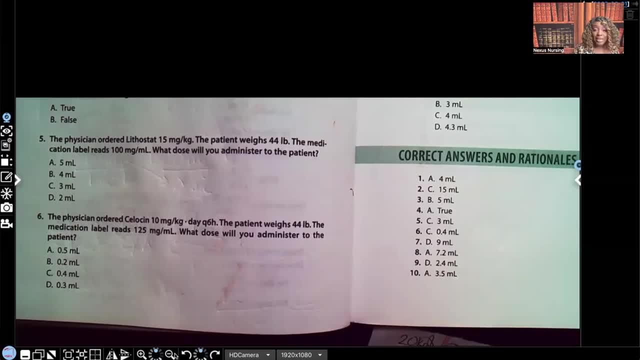 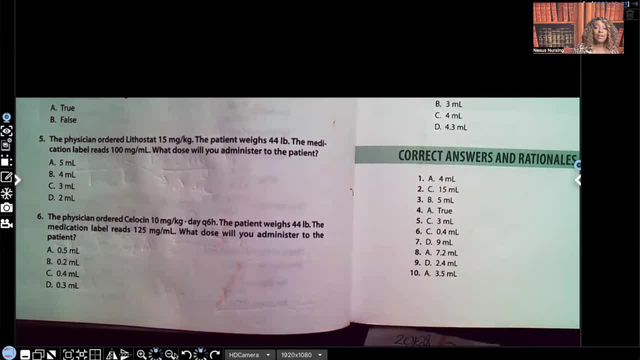 This mistake that I made. this is the biggest mistake that students make. You guys know the math. You will get the answer correct, but you'll forget. after you figure out how much to give the patient per day, you'll forget to change it to how much you're going to give them per dose. 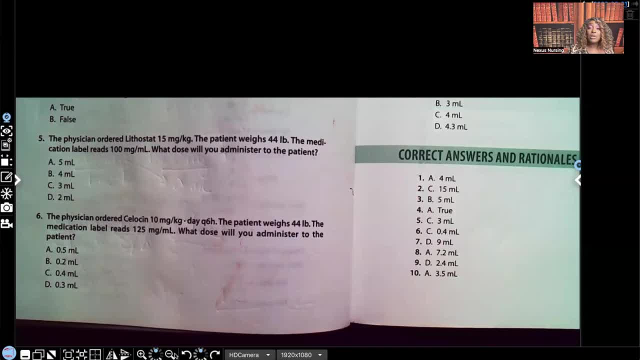 Day is the accumulation- how much you're going to give them within that 24 hours- And dose: Dose is how much you're going to give them every single time that you give that medication. Big difference, All right, guys. I know this was a short video, but for what it was, please let me know what you thought about this video in the comments section.